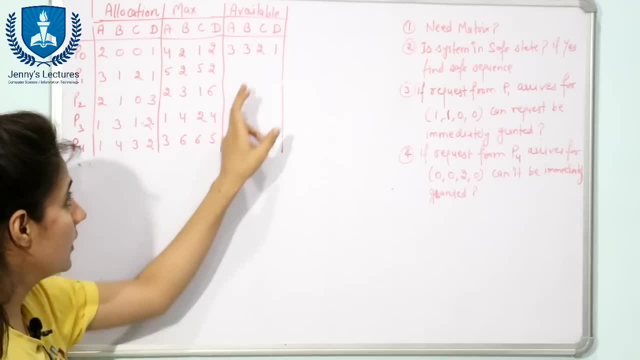 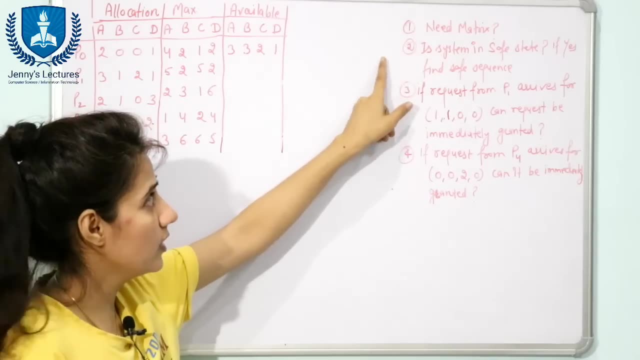 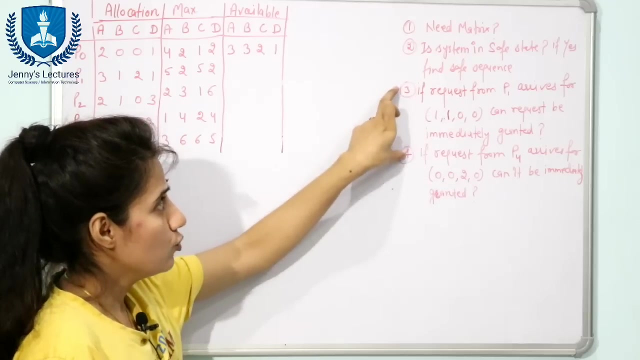 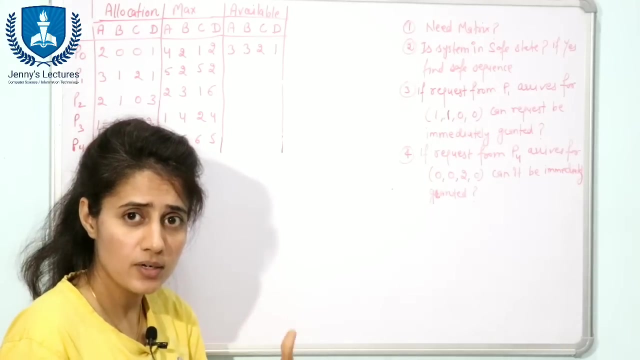 This snapshot is given maximum and allocation and available. we have available resources. we have. and you have to answer these questions. First of all, find out need matrix. Second one is: you have to find out a system in safe state and if yes, then you have to find out safe sequence. Next is see- these two things are new. If request from any process, request from P1, arrives for these resources, can this request be granted immediately? And next is, if request from P4 arrives for this resources, then can this request be granted immediately. 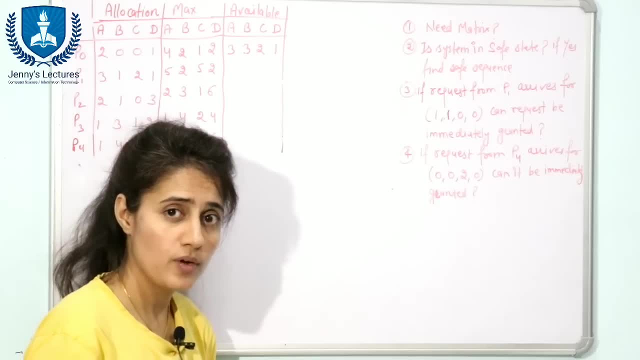 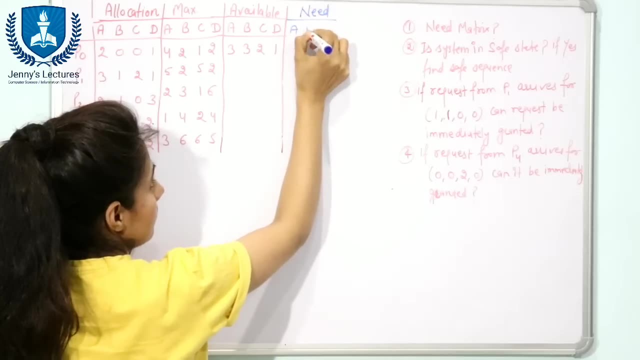 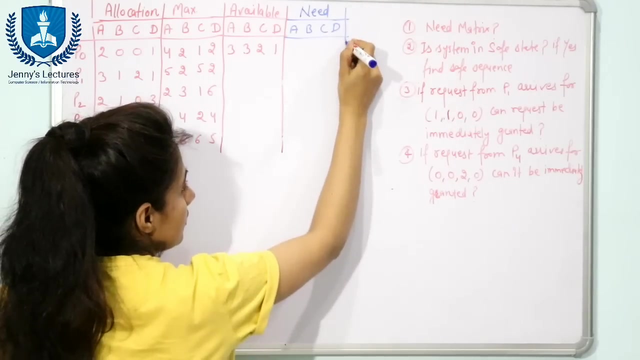 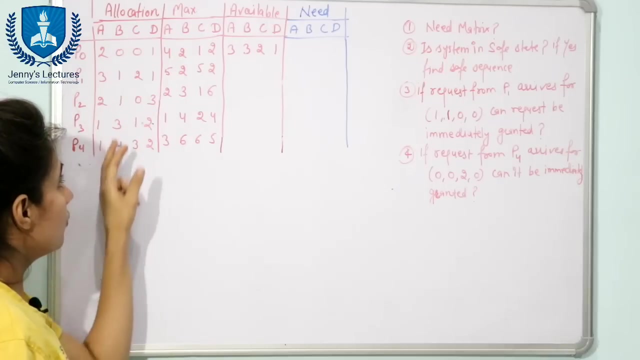 Can this request be granted immediately? We will check out this thing also. So first of all, find out need matrix, Need matrix. how to find out: need matrix, That maximum for that process minus allocation of that process, because each process has already told the operating system that I will need maximum these number of resources and these number of resources are already allocated. So obviously need would be maximum minus allocation. 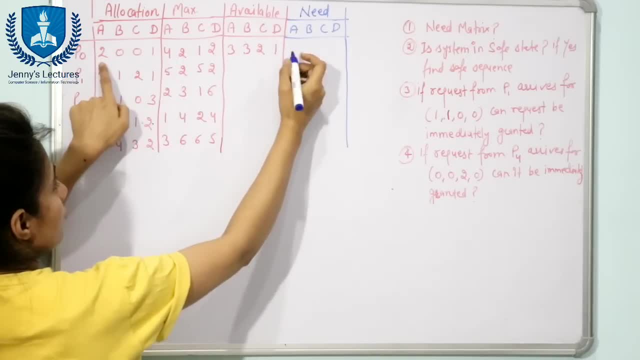 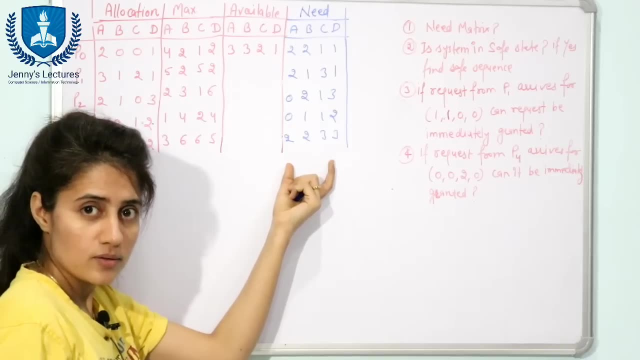 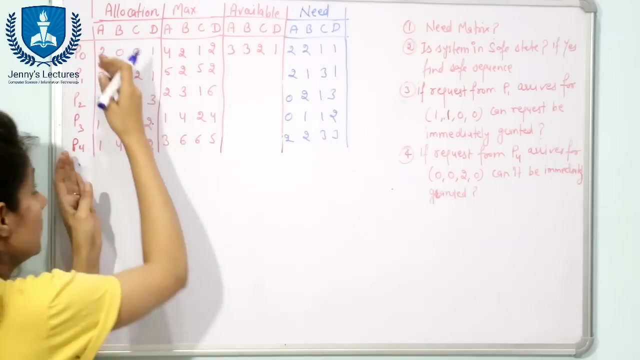 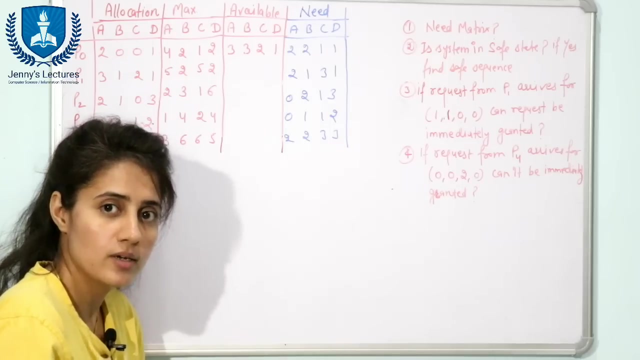 So need matrix of this P0 would be maximum: 4 minus 2 is 2.. Here we will write: 2, 1 minus 0. 1, 2 minus 1 is 1.. So this is the need matrix. Fine, Now next question is: you have to find out a system in safe state. What do you mean by safe state? If the system is able to execute all the processes without going to unsafe state, then you can say: system is in safe state And in which sequence the system will execute these processes. that sequence will be executed. 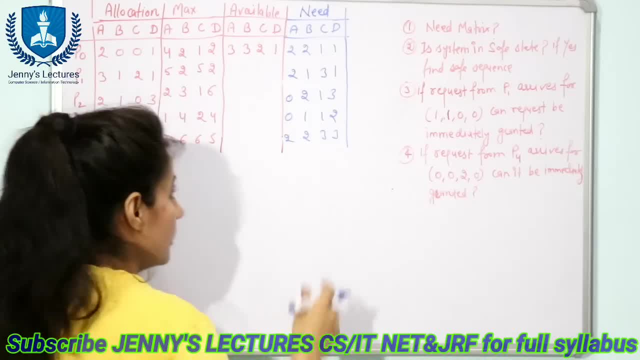 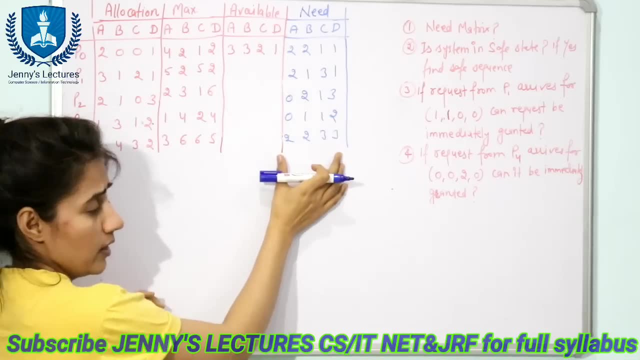 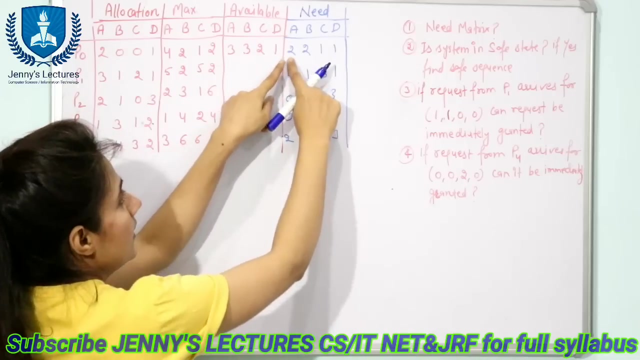 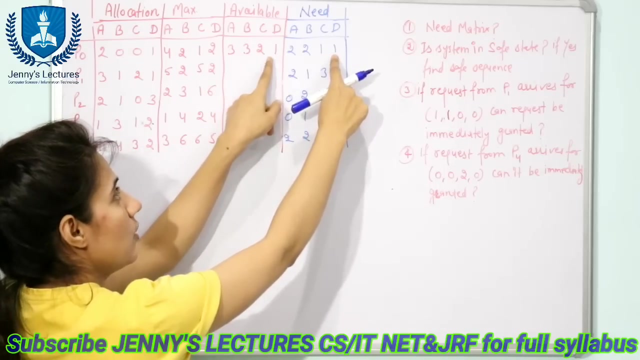 Will be known as safe sequence. Fine, Now find out safe sequence. Currently available resources. are this one? Check out which need you can fulfill, Which process need you can fulfill with this available resources. We will start from P0.. It needs 2 instances of A: we have 3.. It needs 2 instances of B: we have 3.. It needs 1 instance of C: we have 2.. It needs 1 instance of D: we have 1.. Yes, We can fulfill this need. Fine, Now we will write P0. 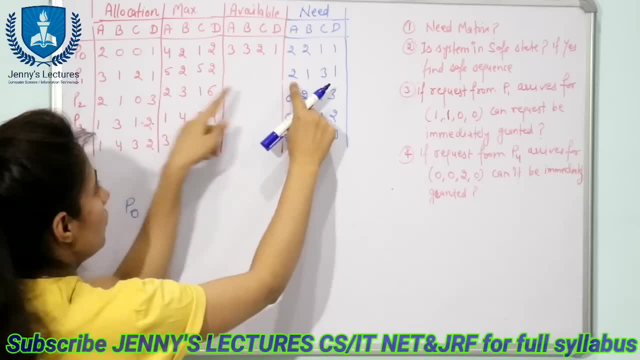 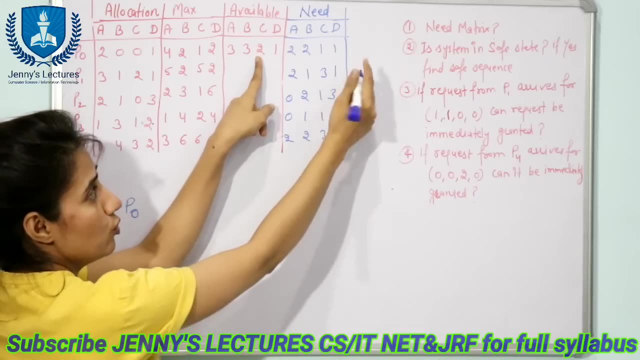 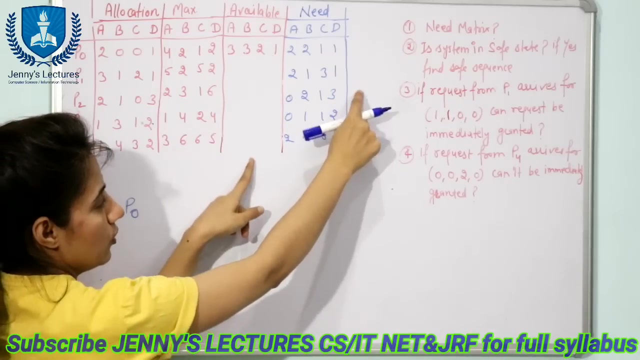 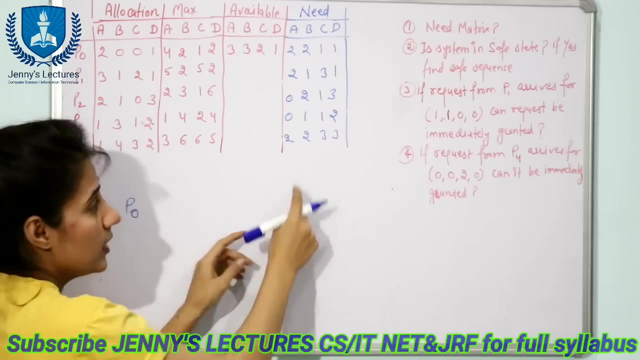 If you want, you can check it out further. For P1 also, It needs 2 instances- we have 3.. It needs 1 instance of B- we have 3.. It needs 3 instances of C, but we have only 2.. So you cannot fulfill this need. Same with this one. See, it needs 3 instances of D, but we have only 1. You cannot fulfill this one. So same with next one. It needs 2 instances of D, but we have only 1. We cannot fulfill this one. Same with this one. It needs 3 instances of D and 3 of C, but we have 2 and 1.. So you can check it out further. 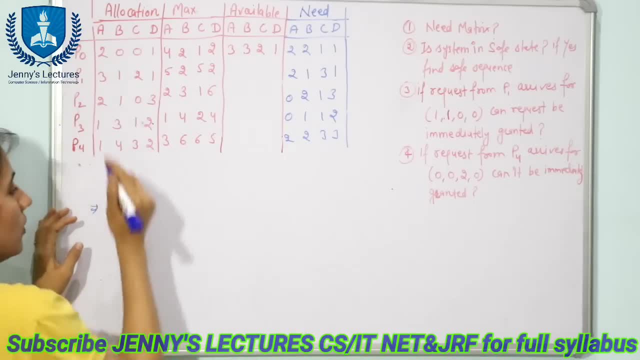 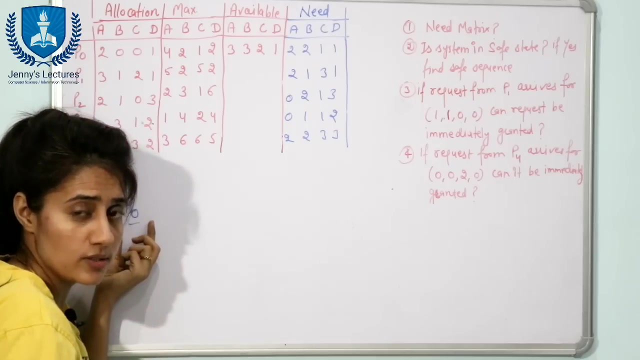 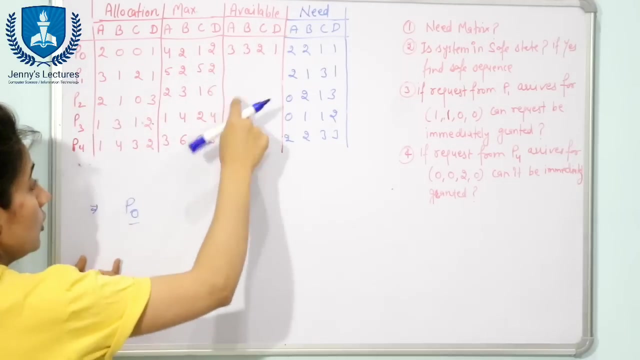 We cannot fulfill this one. The system can only fulfill request of P0.. Second thing: what we will do: Just add the allocation of that process to this available, Because as soon as this process will get all its required resources, then after some amount of time it completes its execution and then it will release all its allocated resources. So what you will do in available resources, just check out the allocation of P0 and add to this one. 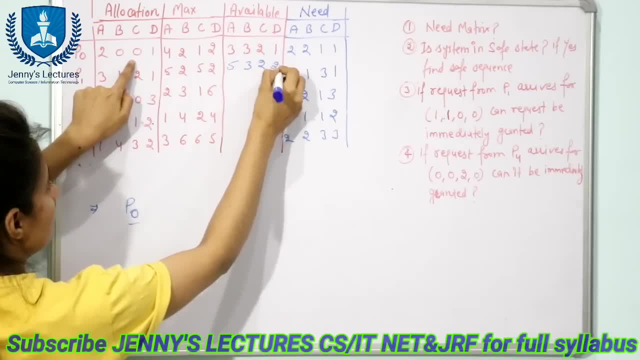 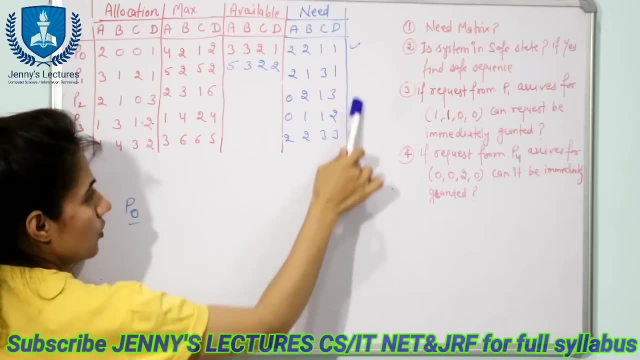 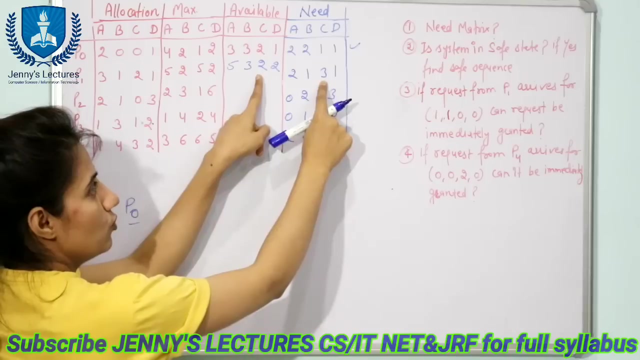 3 plus 2 is 5.. Here 3,, here 2, here we have 2.. Now, this P0 got completed. Now, with the help of this available resources. now which process need you can fulfill? Check out For this: one: 2,. we have 5,. 1, we have 3.. It needs 3 instances, but we have only 2.. So you cannot fulfill this need. 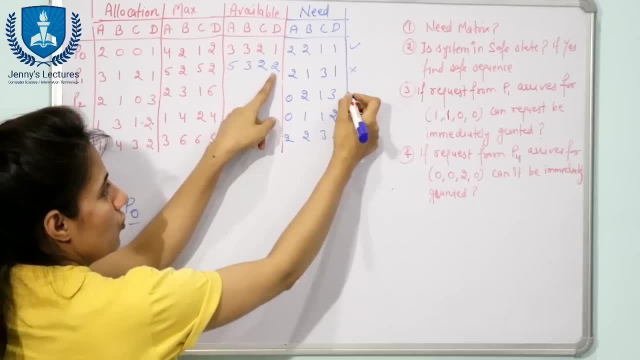 What about this one? It needs 3 instances of D. we have 2.. You cannot fulfill this one. What about this one? Yes, we can fulfill this one. It needs 0, 5.. It needs 1, we have 3.. 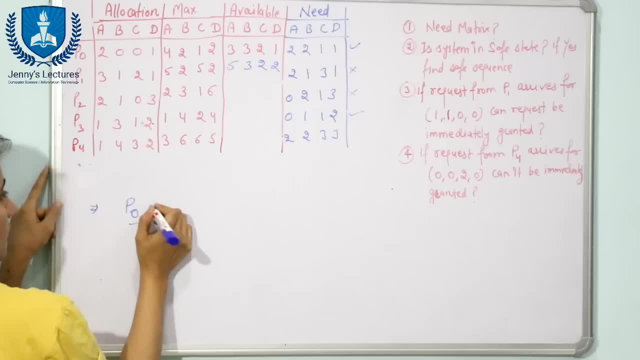 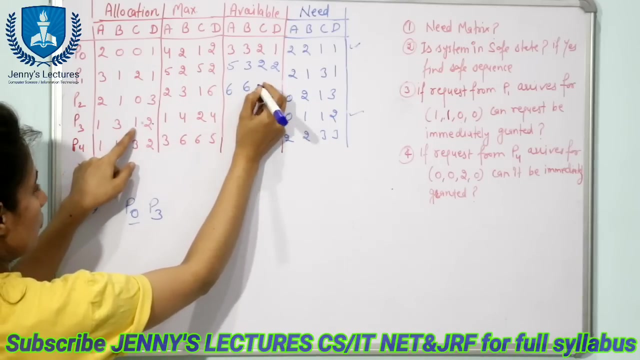 It needs 1, we have 2.. It needs 2, we have 2.. So you can fulfill this request. So next is P3.. Fine, Now next thing is just check out the allocation of this P3 and add in the available resources. 5 plus 1 is 6.. 3 plus 3 is 6.. 2 plus 1 is 3.. 2 plus 2 is 4.. 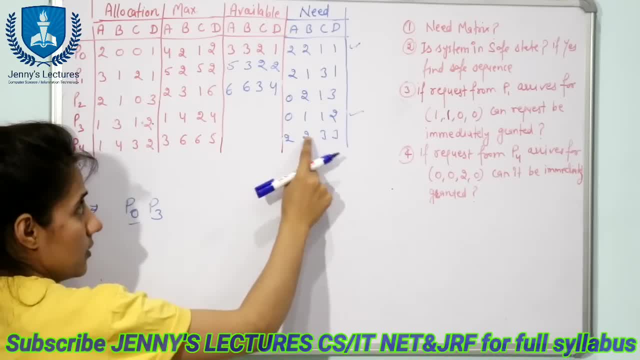 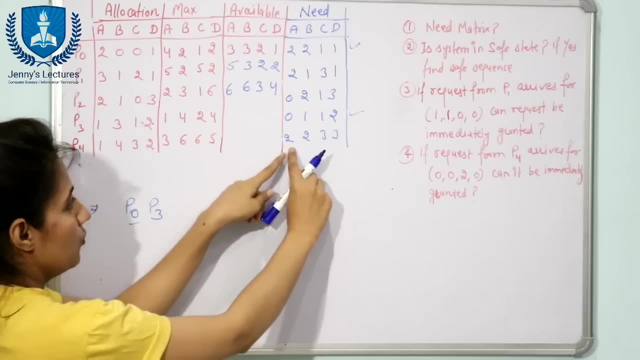 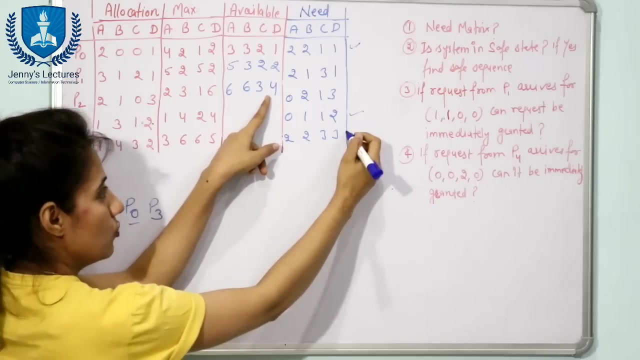 Now, P3 also got completed. Now remaining is 3. Check out with the help of this resources. Can you fulfill request of any of these 3?? We will check out with P4.. It needs 2.. We have 6.. It needs 2.. We have 6.. It needs 3 of C. We have 3.. It needs 3.. We have 4.. Yes, you can fulfill this need. 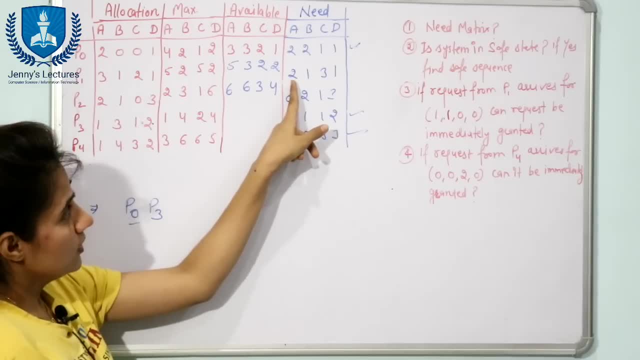 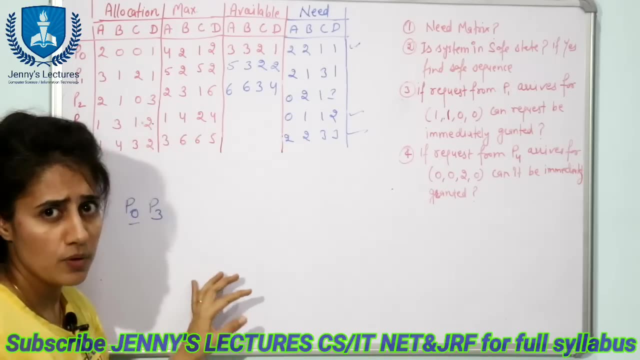 You can check it out for this also. Fine, See this need also we can fulfill with this available resources. So either you can execute P0 or either you can execute P1.. So save sequence can be more than 1.. It's up to you how to solve this question. 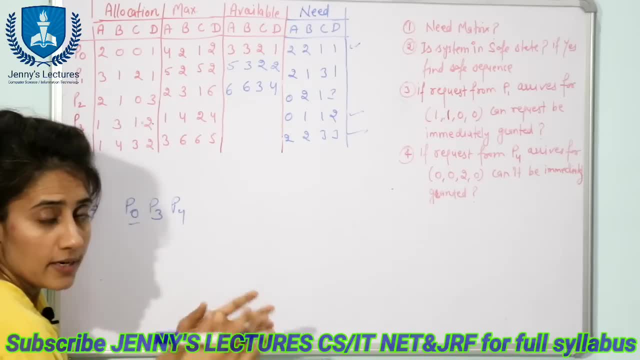 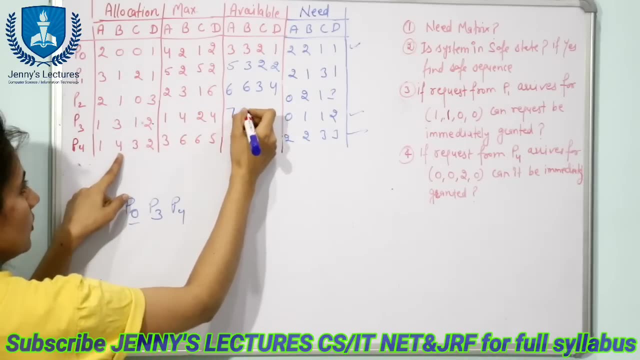 Next is P4.. Now P4 got completed and it will release its resources, So we will add its allocated resources to available sources. now, 6 plus 1 is 7.. 6 plus 4 is 10.. 3 plus 3 is 6.. 4 plus 2 is 6.. Fine. 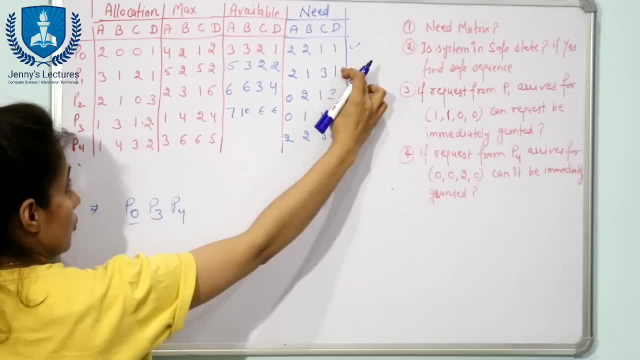 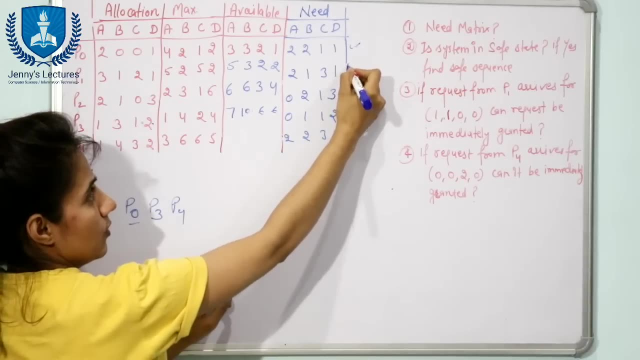 Now next is we have these 2 resources. So obviously I guess with these resources you can fulfill this need also and this need also Fine. So either you can take P1 or you can take P2.. Suppose I am taking P1.. 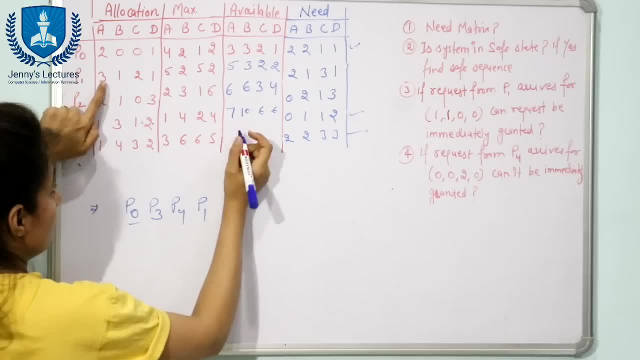 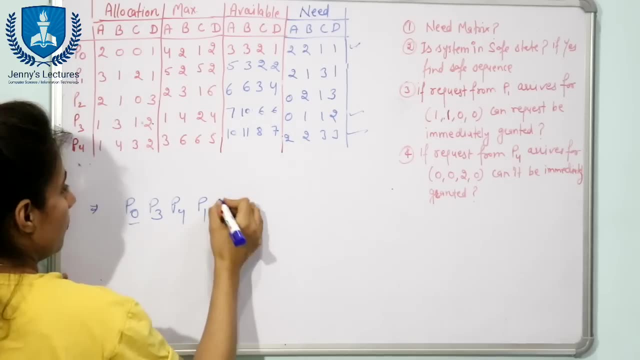 Now add the allocated resources of P1.. Now add P1 to this. available resources. 7 plus This one is 11.. Fine, Now finally, we have P2.. Now check out allocation of this one and add to this one 10 plus 12,, 12,, 8 and 10.. 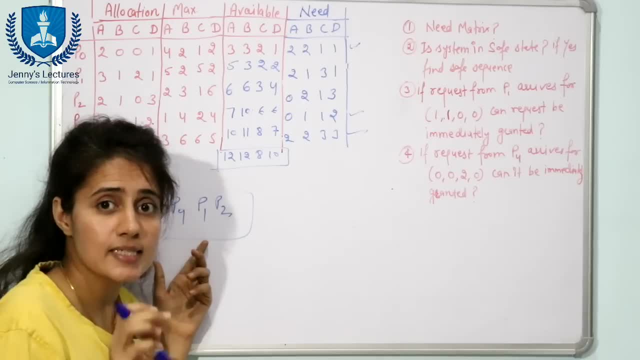 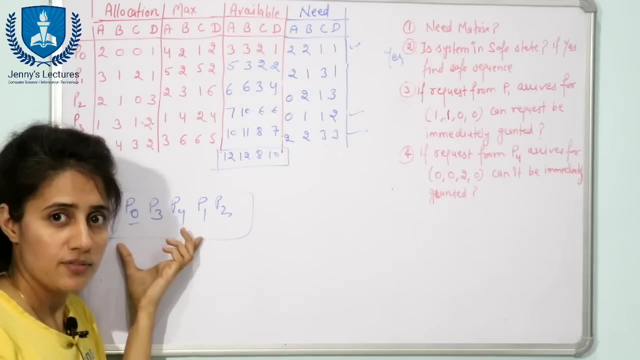 So you are able to find out a save sequence. It means system is in save state. So answer would be yes. And what is save sequence? So this is the save sequence. See, save sequence can be more than 1.. Fine, So I got this save sequence. 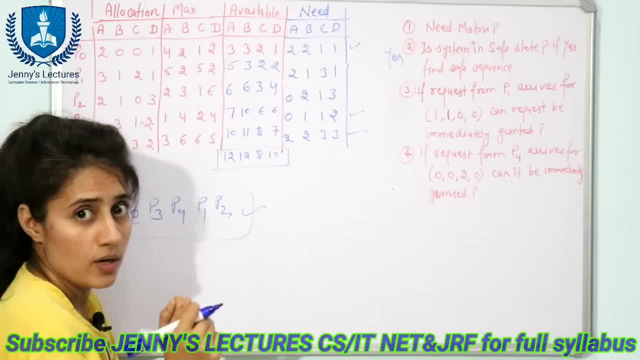 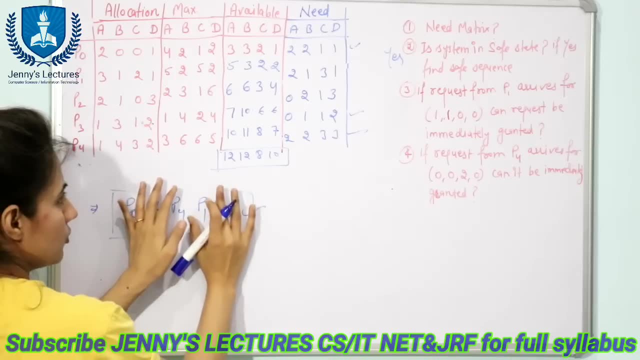 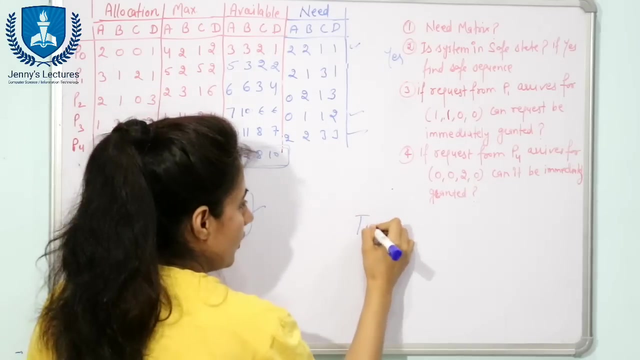 Fine, Now see, you can check it out. You can tell your answer. How available resources are this one? and after executing all the processes, you got these number of resources. It means total number of resources are this one? Fine, Now how to find out total number of resources. 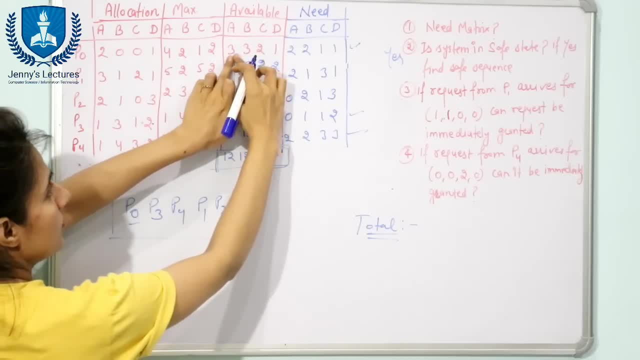 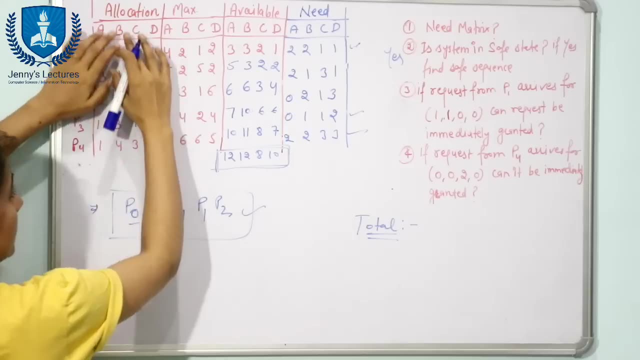 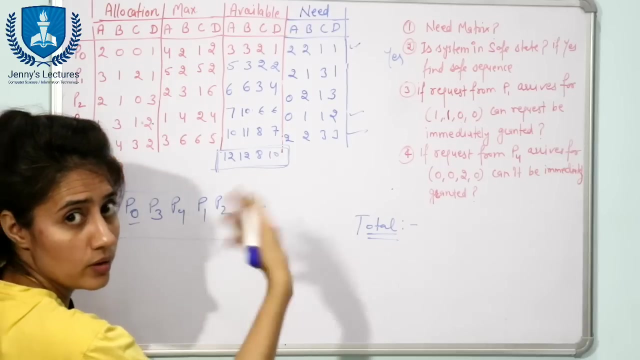 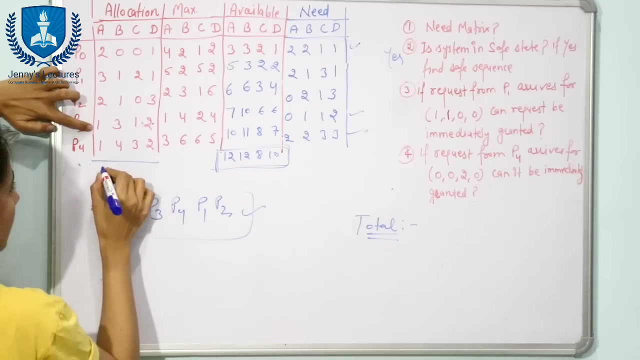 Now see First of all, at first, available resources were this one and after allocating these resources, these were available resources. So just add the allocated resources plus these available resources and you should get this number. Then you can say that you are going right. So just add these resources, These allocation resources, 2 plus 3,, 5, 7, 9.. 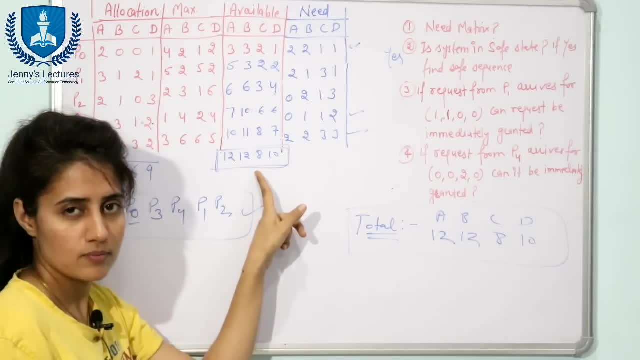 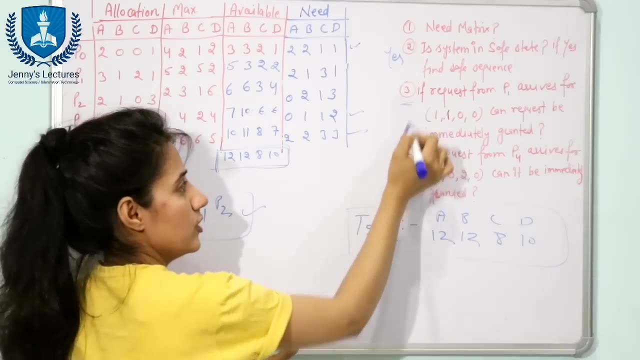 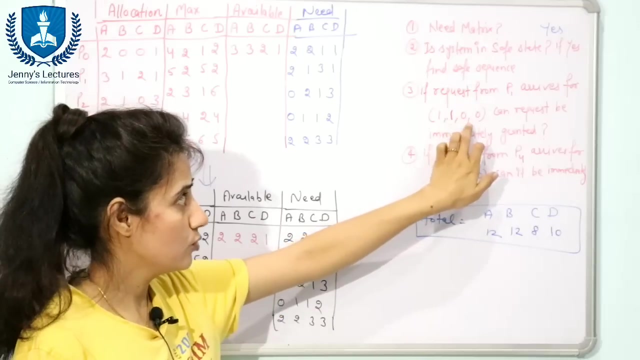 See now: this and this number is same, So you can tell your answer like this also. Now we will discuss how to solve this question. So now the third question is: see if any request from P1 arrives for these number of resources, then can this request be granted immediately? 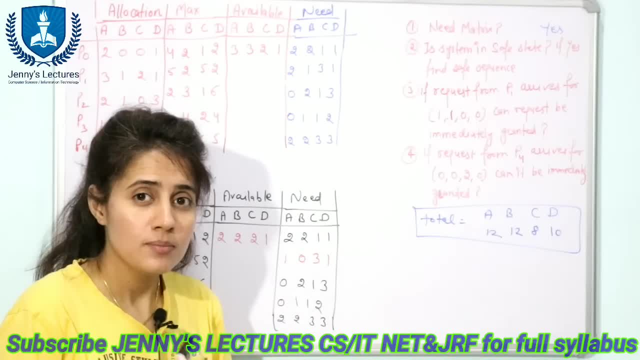 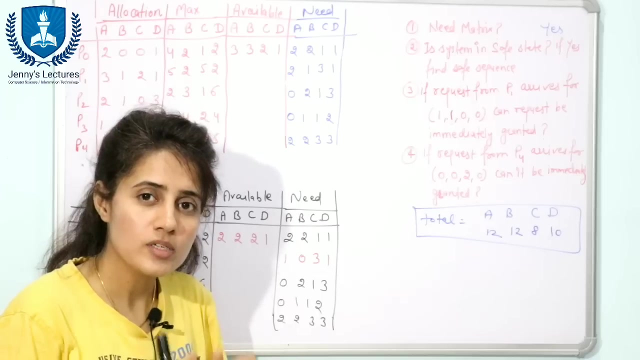 Fine, See, when a request comes, then the system does not grant that request immediately in deadlock avoidance case. Why? Because deadlock avoidance case is futuristic approach, So system will at that time will not grant that request immediately. system will check if, if i request. 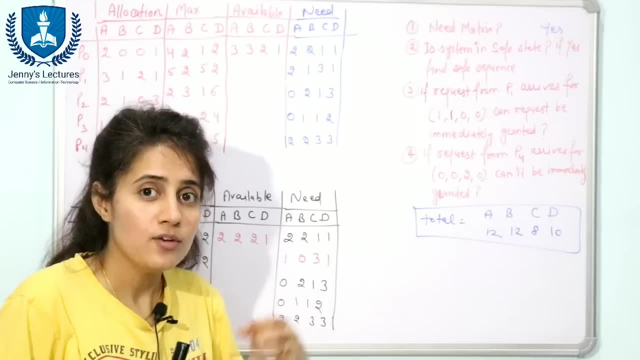 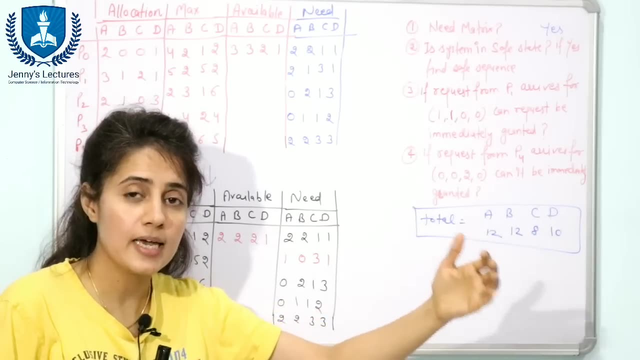 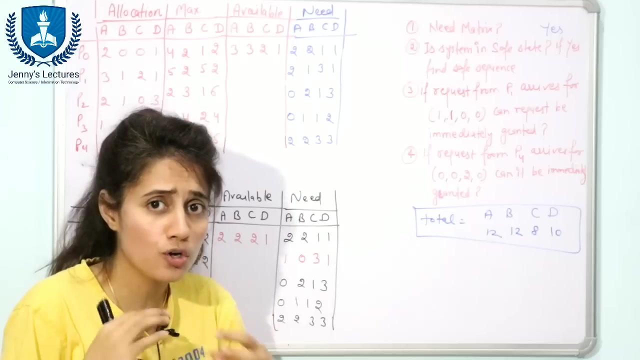 if i grant this request at this time, then will i be in safe state in future or will i get any deadlock in future? so if that system get any deadlock, maybe immediately because of that request or maybe in future, then that request would not be granted at that time, although the resources 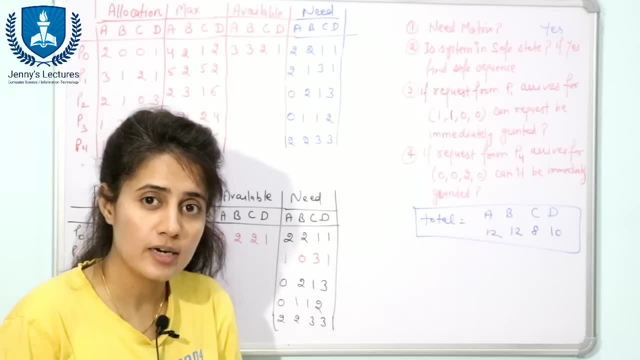 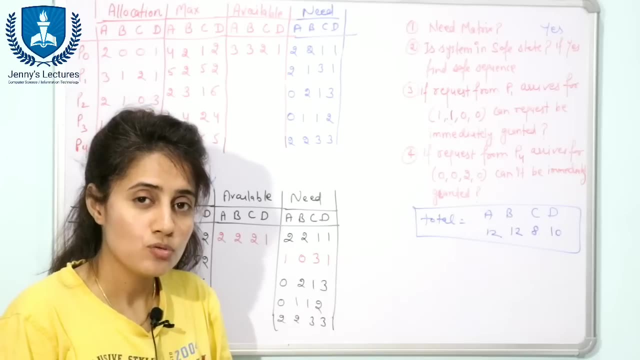 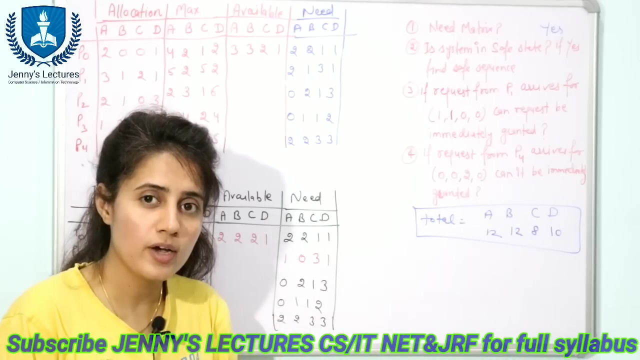 are available, but that in that case also system will not grant that request. why so? because it analyzed that it has some data and it analyzed that data and it it comes to the point that because of that granting of this request at this time, i can get deadlock in future. so that is why. 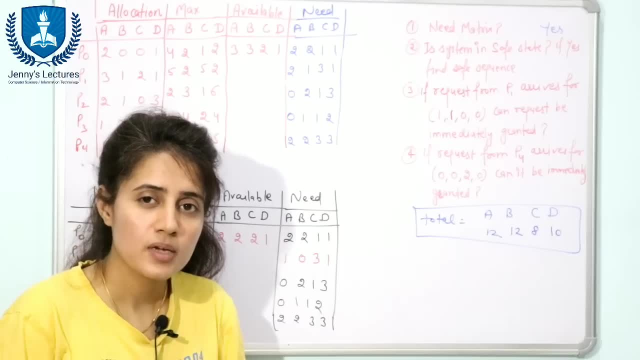 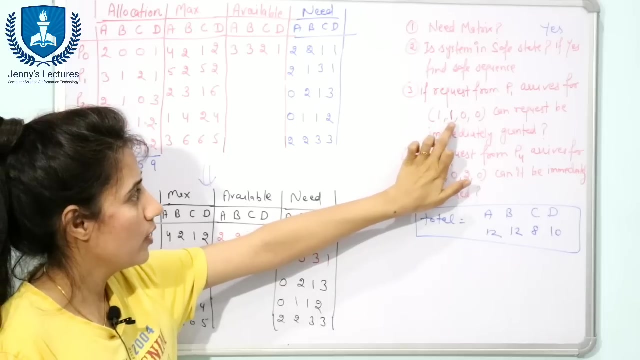 that system will not. that request will not be granted. now how how this would be checked. this would be checked using the source request algorithm and then finally apply the safety algorithm or you can say bankers algorithm. so now check: p1 is requesting for resources 1 1, 0, 0 and we have this snapshot. need of this matrix. 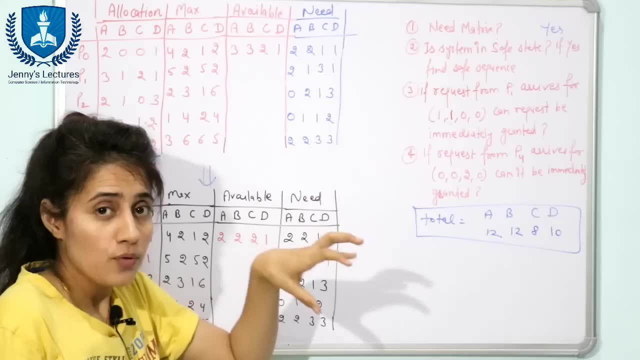 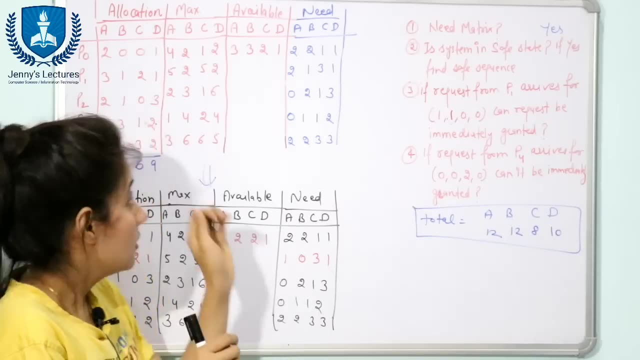 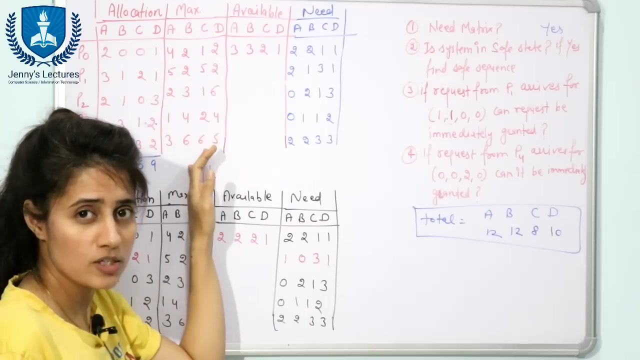 now. so i hope you know that that p1 or any process cannot request more resources than its need matrix, because each resources, each processes, has initially told the system that we will need maximum these kind of resources. so now check: p1 is requesting for resources 1 1, 0, 0 and we have this snapshot need of this matrix. 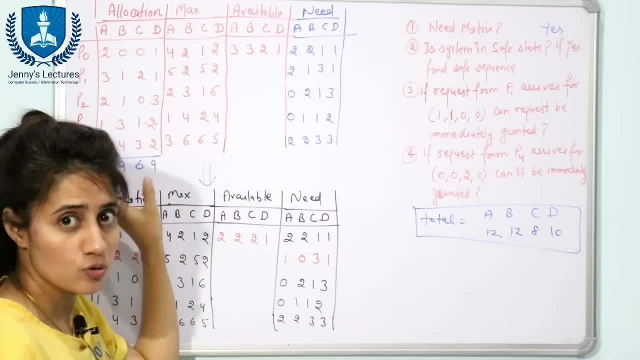 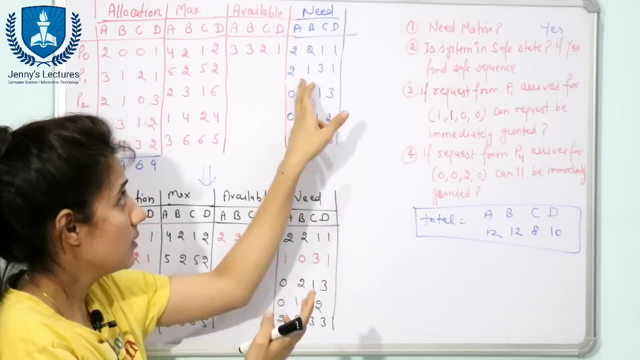 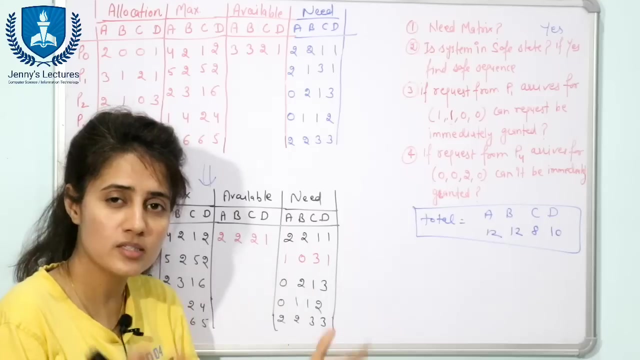 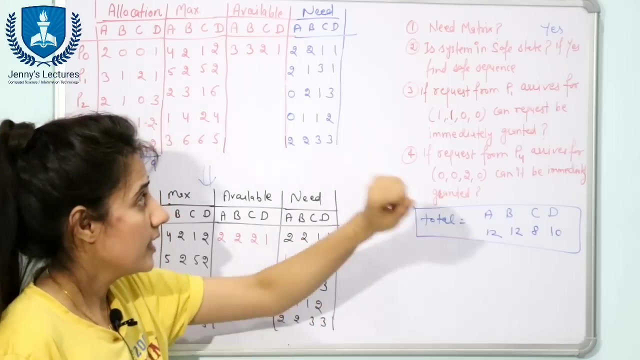 and at this point of time already allocated resources are this one. so obviously that process, the need matrix, will calculate and that process can now request this, these number of resources at mix. so if this request is exceeding from this need matrix, then the system will raise an error that that process has exceeding its claim. fine, and second thing is we will check. 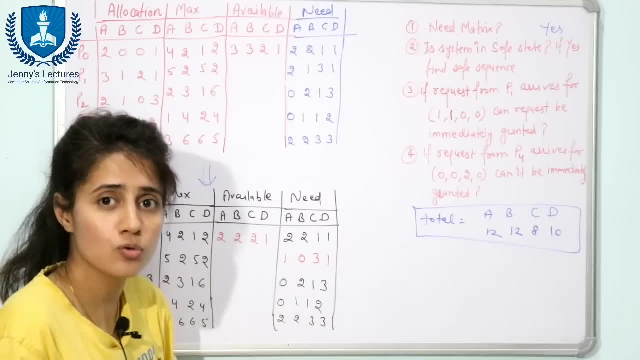 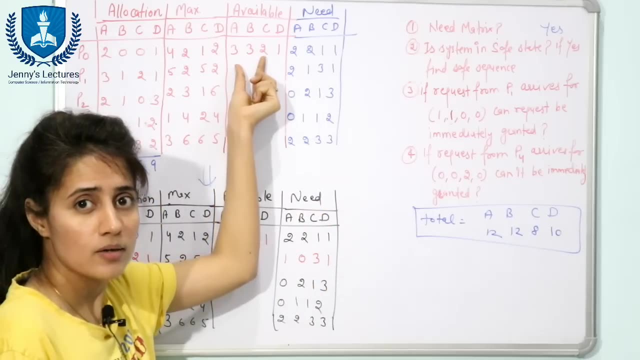 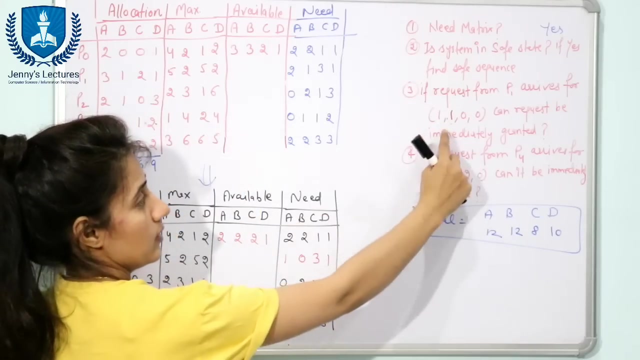 if this request, we have this number of available resources or not, and we will check if this request should be less than or less than or equal to available resources. fine, now, if this is true, now see this request is: p1 is requesting 1, 1, 0, 0. so this the need matrix of p1 is 2, 1, 3, 1, so obviously this. 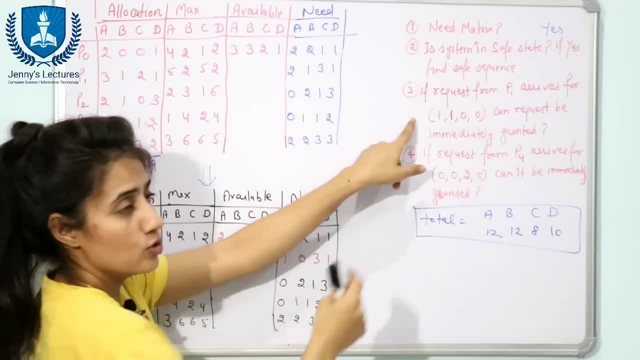 1 is less than 2 and 1 is less than. 1 is less than or equal to 1. so first condition is true. now we will check do we have the available resources or not to fulfill this request. so check out our available resources and we will check. this request should be less than or equal to available resources. 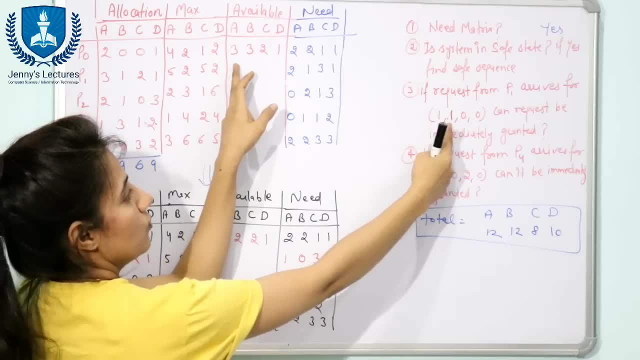 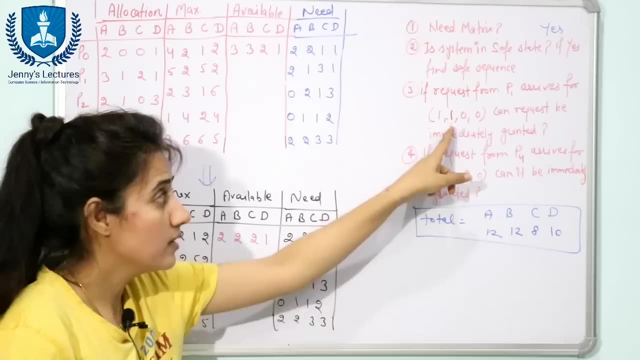 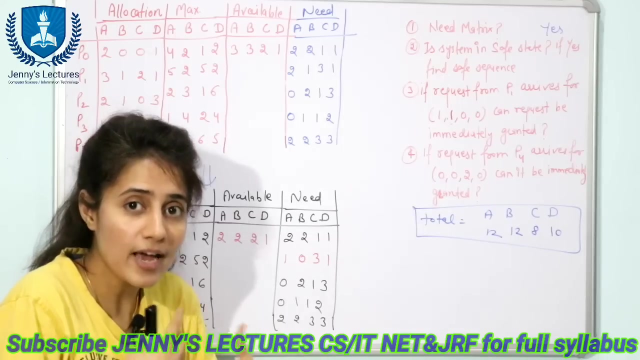 one instance it need we have three. one instance it need. we have three instances of way. yes, we have these kind of resources, but it doesn't mean that system will grant this request immediately. no system. third step is: system will pretend not actually grant that request, but system will. 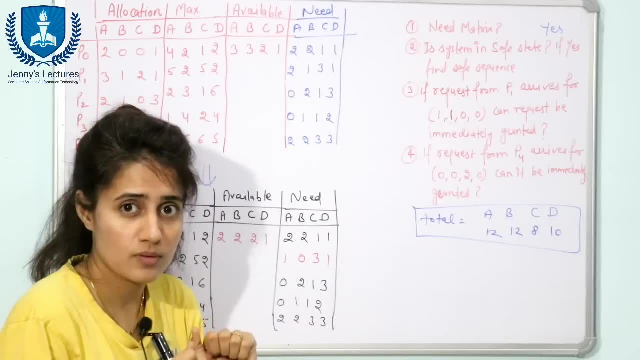 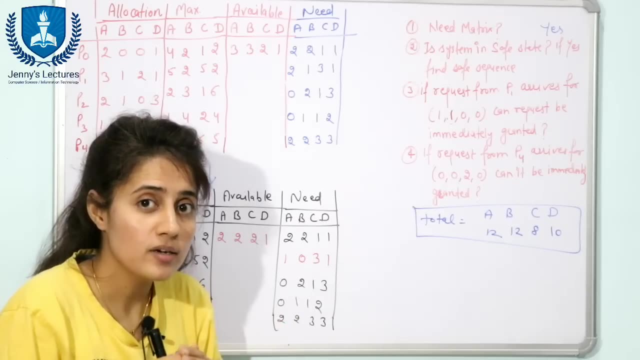 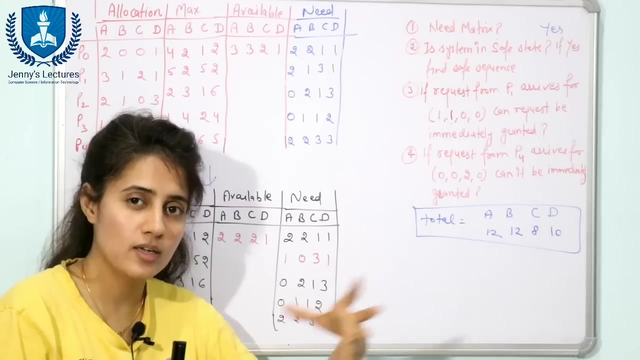 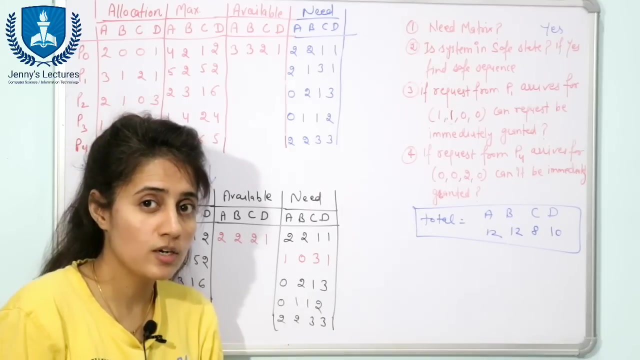 pretend as if it has granted this request, fine, and then it will check, it will apply bankers algorithm or it will apply that safety algorithm and check in future. if it is able to find any safe sequence, then we can say that that's then the system will grant that request. if the system will go in unsafe state because of this request, then it 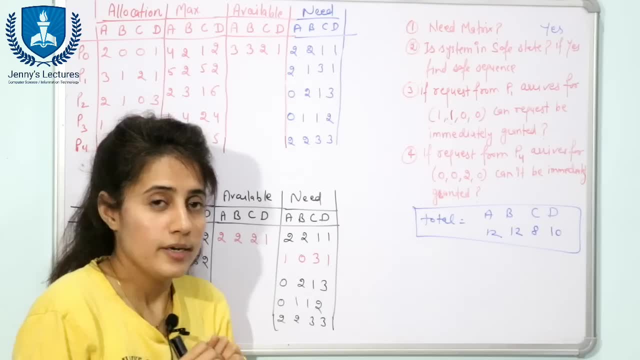 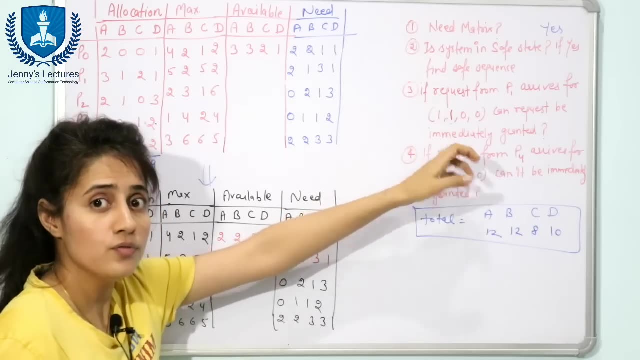 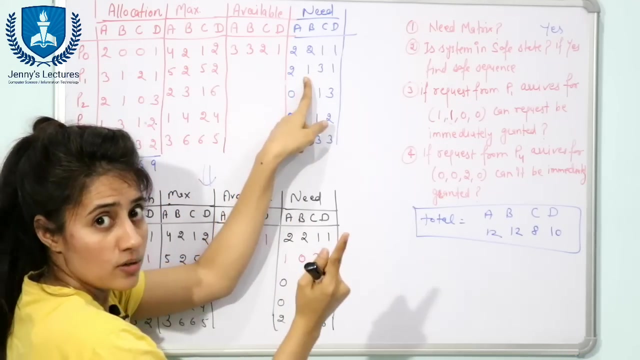 will not grant this request. fine, now, see you now. system at this point, system are pretending that it has granted this request. now, if system grants this request, then what will happen? obviously, the need matrix of this p1 will be changed. need matrix would be this: need matrix minus this one. 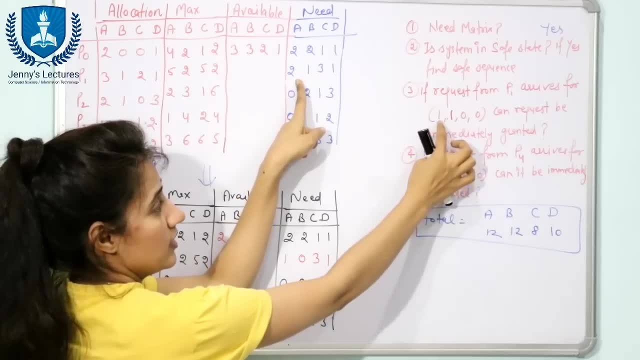 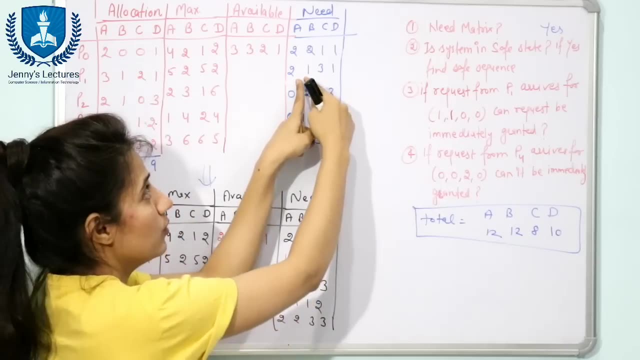 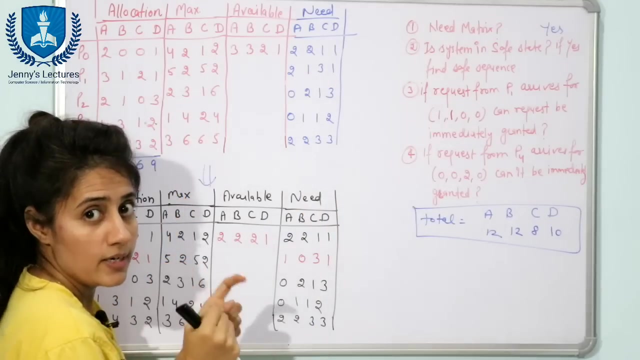 fine, because p1 has recrested this one and system has allocated this. system is pretending that it has granted this request. so need matrix would be: need matrix minus this one: 2131, so 2131 minus 1100, now, second thing: what would be updated is this available matrix, because system has, system is has. 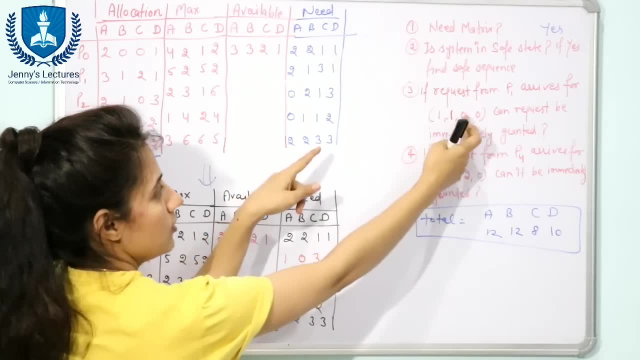 15Guger bit of selection. what will be of fast, normal, automatic allocation system is process is fine. system needs matrix will be need matrix minus this one. 213121212. rhythm should be noted as we can see here, granted this request, so obviously the this 1100, this request would be detected from. 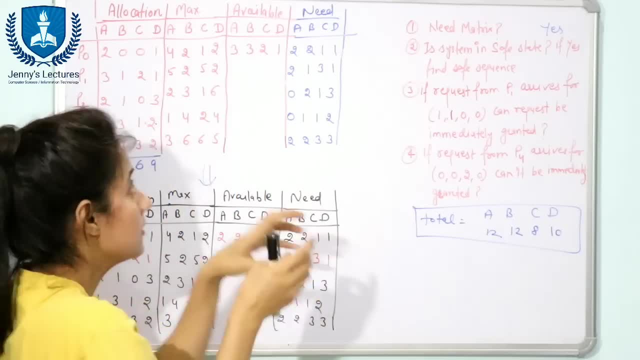 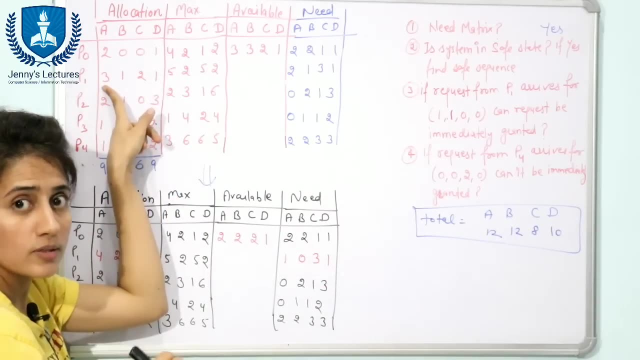 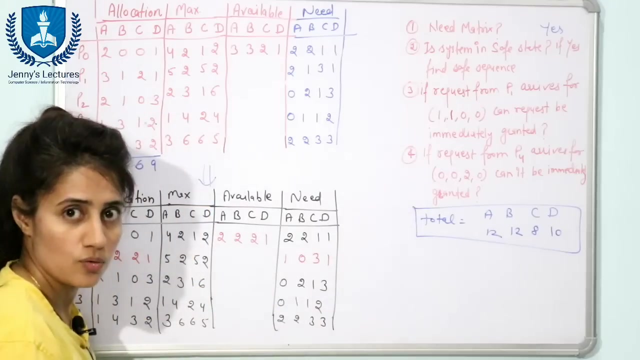 available resources. and third thing is already allocated resources are 3121 and again this number of resources would be allocated to this matrix. then the allocate allocation of this p1 would become this allocation plus 1100. so after updating these three changes, then this, this state. 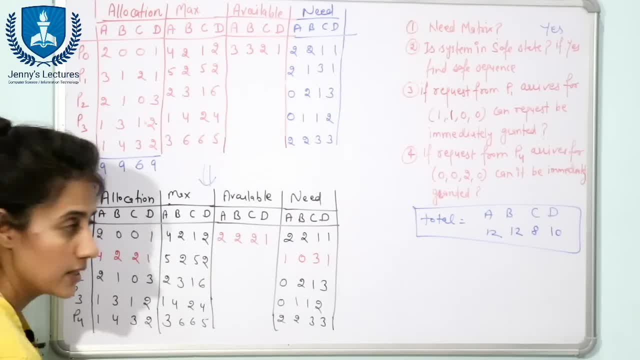 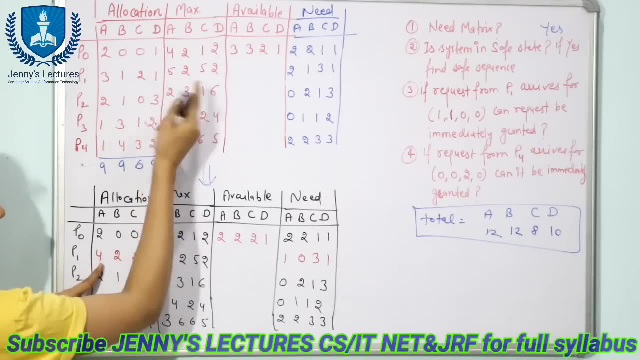 of the system will be modified to something like this: see, everything is same, only we have updated three things: the allocation of p1, 3121 plus this one, 3 plus 1 is 4, 1 plus 1 is 2 and 2: 1. next we. 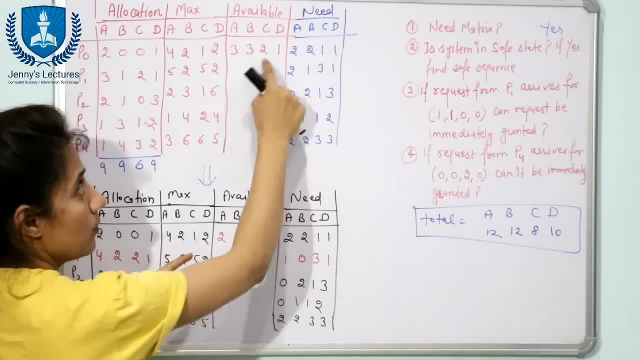 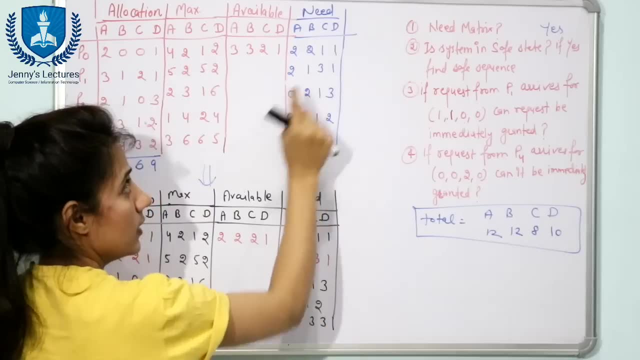 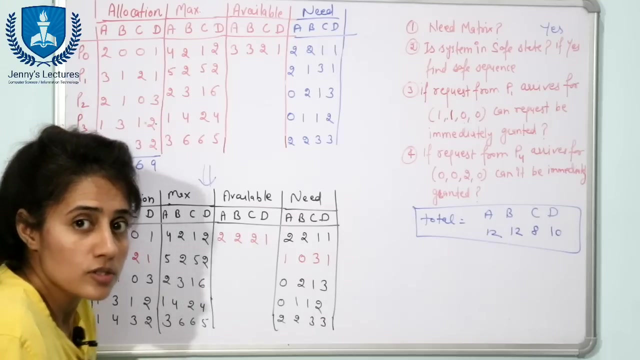 will do: we will update this available. we will minus these number of resources from this available. so this would be available. third thing: what you will do, you will minus this resources, this request, from need matrix. so this would be something like this and all thing would be same. now system system would apply this safety algorithm and system. 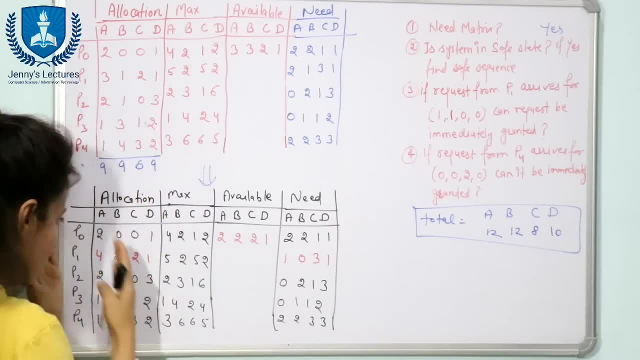 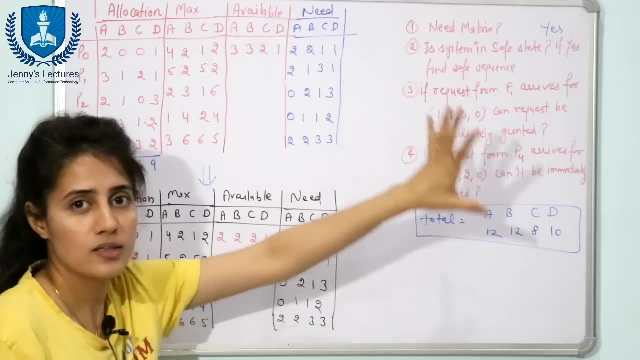 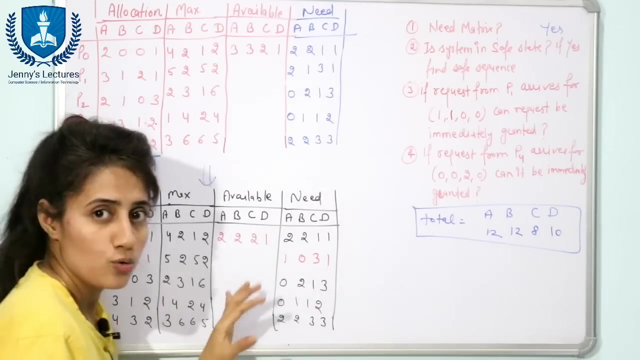 will check, will I am? will I be able to execute all these processes safely? and if yes, then since then system will grant this request. now, system is pretending, system is checking for its future. so now, at this case, now, at this snapshot, apply that same algorithm that bankers. 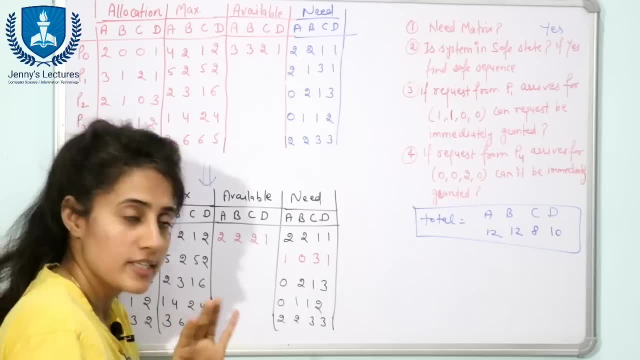 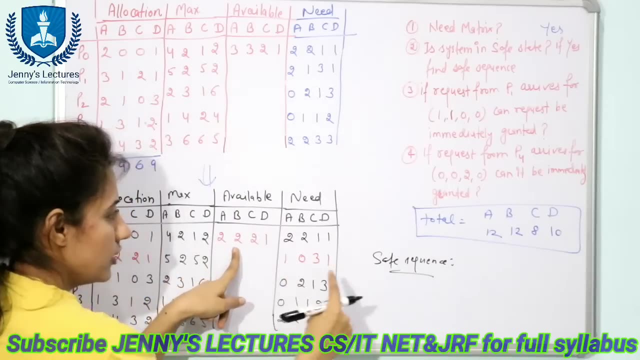 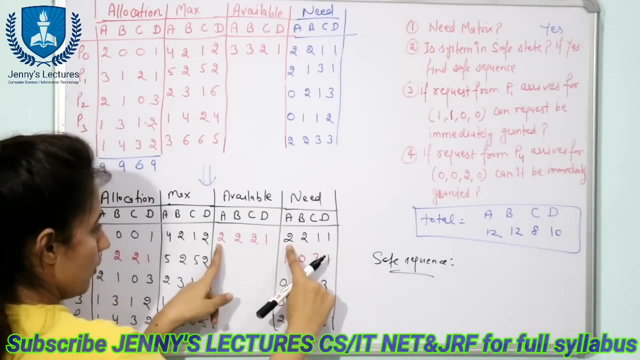 algorithm how you will apply that algorithm. find out safe sequence now. how to find out safe sequence. see with the help of these available resources now. now check: can you fulfill request of any? any process? check it out. this p note requires two. we have two instances. two we have. 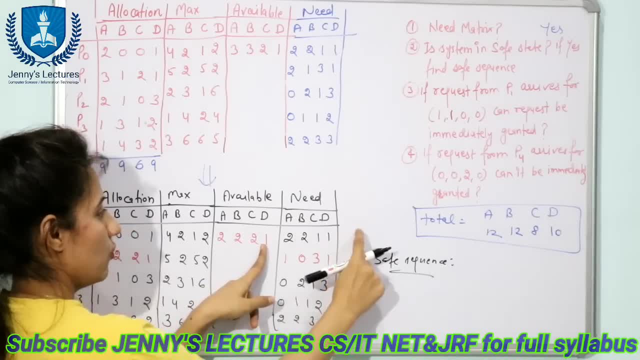 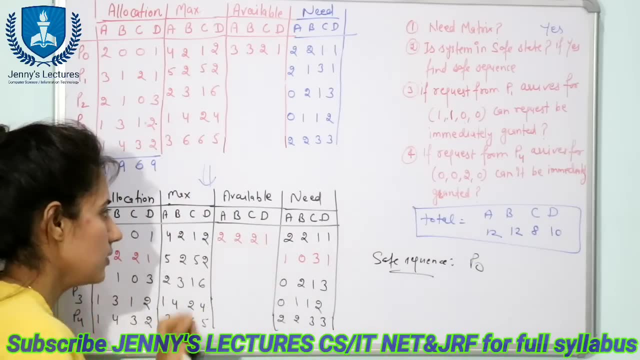 two instances. one we have two instances and one we have one instance, so we can fulfill this request. so see, we will execute p1 first. fine, you can check it out another also, and if you will find if you system is able to complete any other process also, then you can write down that you can start your safe sequence with that process also. 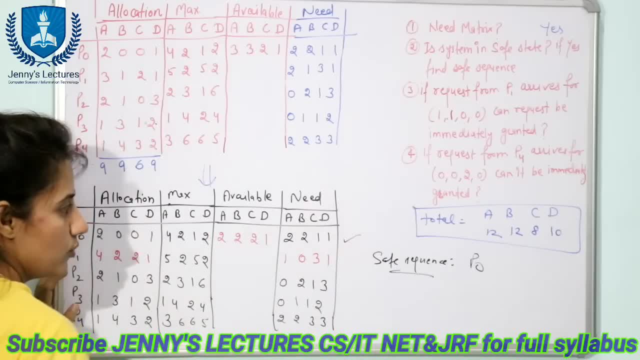 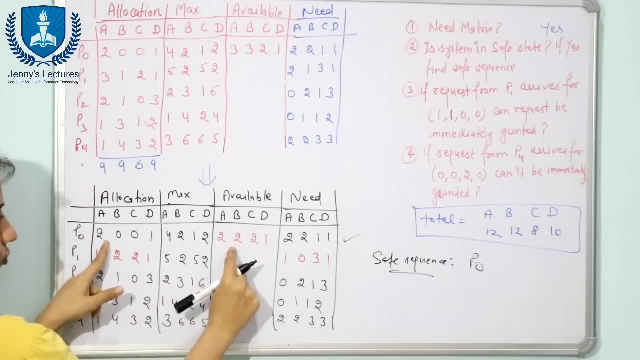 it's fine. now p1 has been executed. now what the next step is what? in banger's algorithm, we will add the allocated resources of this, this process, to available resources, because this p p0 now got completed and it will release all its allocated resources. two plus two is four. two two, two, two two. 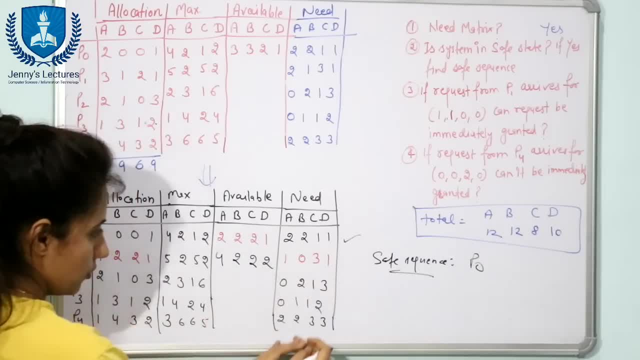 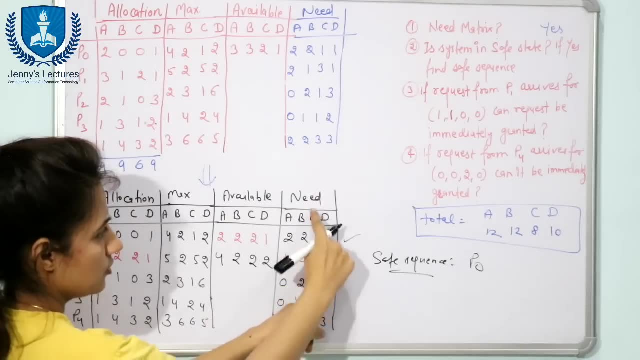 now find out now. next is p1. now check out. can you fulfill this request? no, why so? because it requires three instances of c, but we have only two, so you cannot fulfill this request at this time. now check out this one. see it. it requires three instances of this d, but we have only two, so we cannot fulfill. 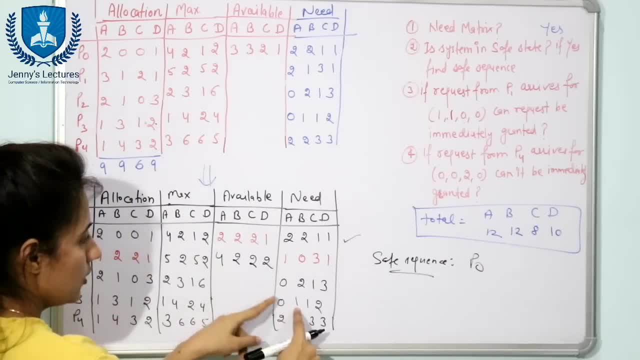 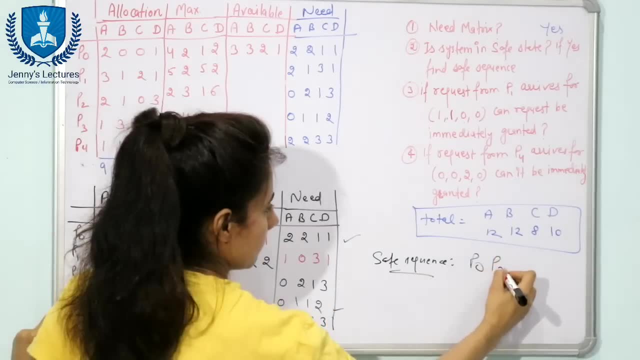 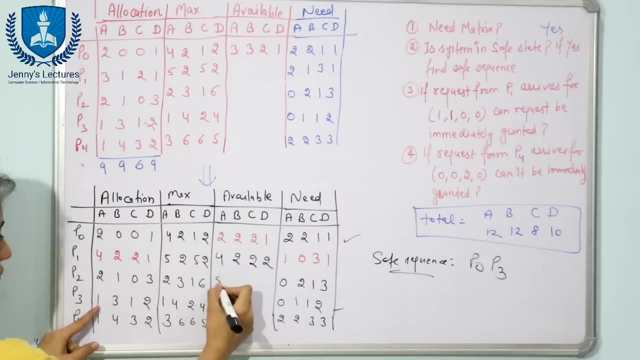 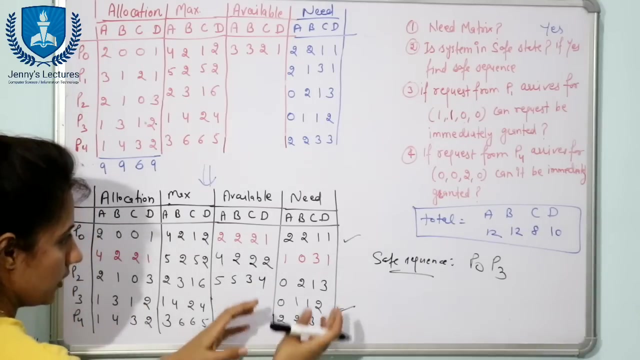 this request. check out for this: one: zero. we have four. it requires one. we have two. one. we have two. fulfill this request. so now p3. now what you will add in available resources, allocated resources of this p3: 4 plus 1 is 5, 3 plus 2 is 5, 2 plus 1 is 3, 2 plus 2 is 4. now this work completed. now find. 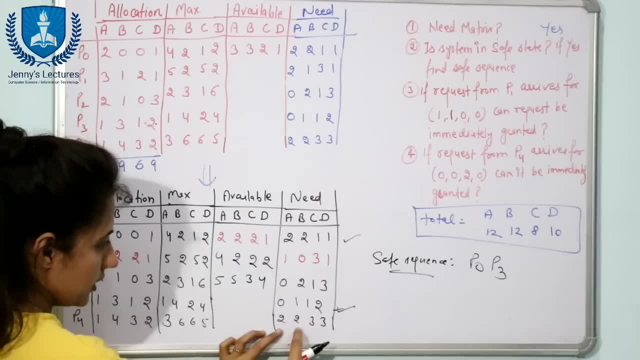 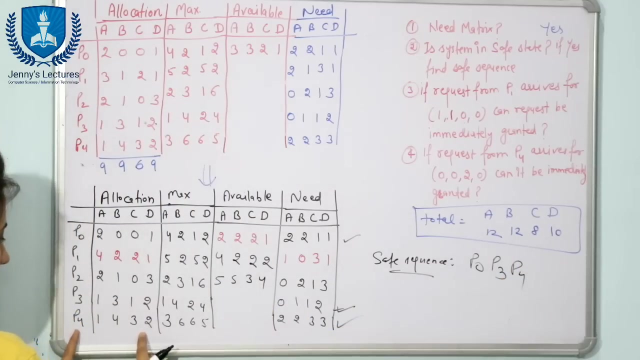 out next. next is p4. can you fulfill this request? yes, we can fulfill 2. it is less than 5. it requires 2, we have 5. it requires 3 instances. we have 3. it requires 3 instances, we have 4, so you can fulfill this request also now. p4. now add allocation. allocation resources of this p4 in. 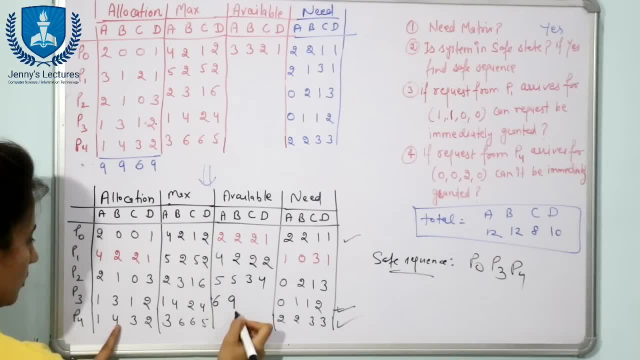 this available resources: 5 plus 1 is 6, 5 plus 9, 3 plus 3 is 6, 4 plus 2 is 6. now p4 got completed. now next remaining is p1 and p2. so obviously, with this help of this available resources, you can. 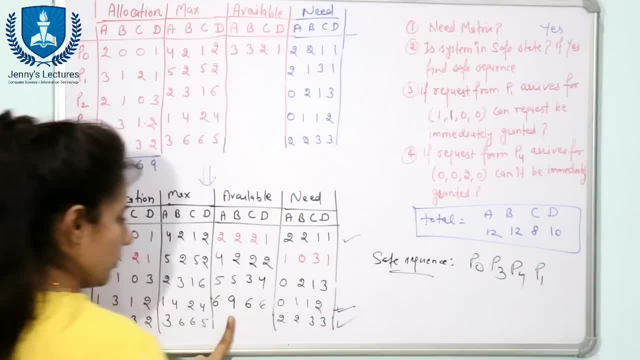 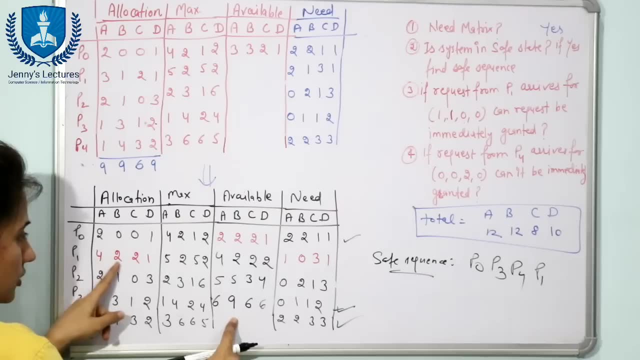 fulfill this request also and this also, so you can take either p1 or p2. i'm taking p1, so after completing p1, we will add the allocation resources of p1 to available resources. now this allocation resources not go for this one, because we have updated this state to this state: now: 10, 11, 8, 7, now p1. 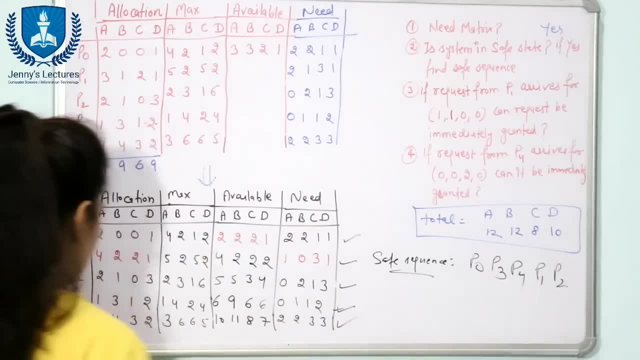 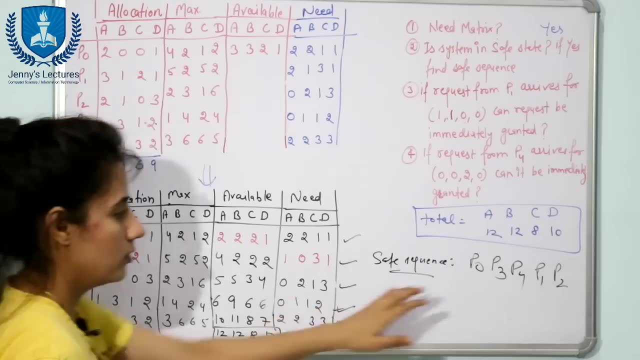 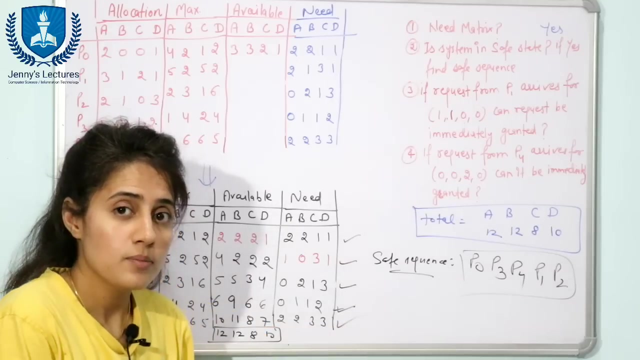 completed now. next is p2: now add allocated resources of p2 12, 12, 8 and 10. now, after completing all the say: this is safe sequence now, system is able to get safe sequence now, system can grant this request. or you can say: system will grant this request now after checking. 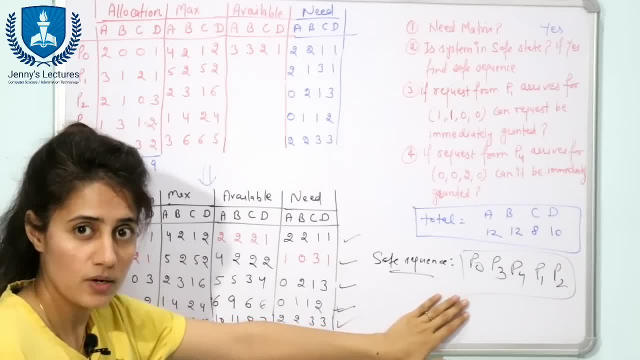 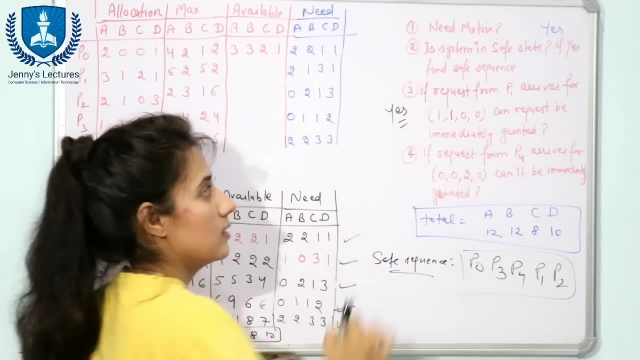 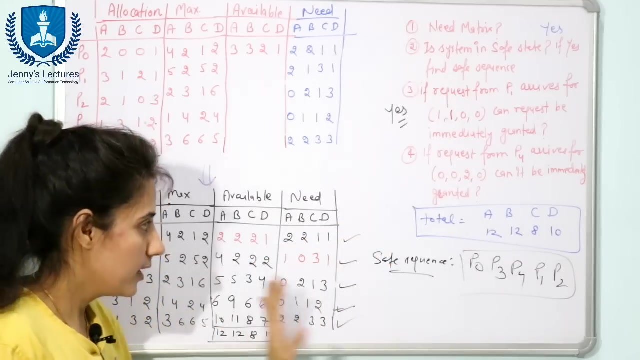 this case, after checking the safe sequence. fine, if system is able to get safe sequence, then system will grant this request. now you can say: yes, this request. can this request be granted? yes, this request can be immediately granted. fine, because after granting this request, system is able to. 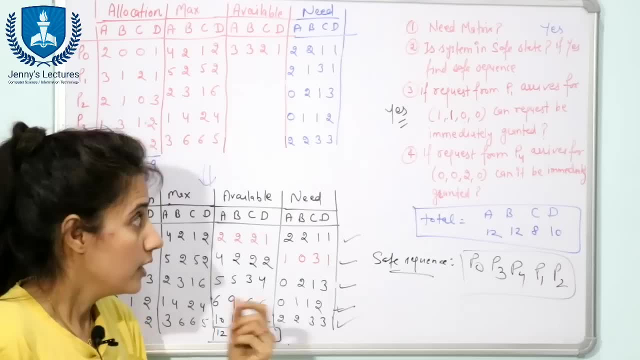 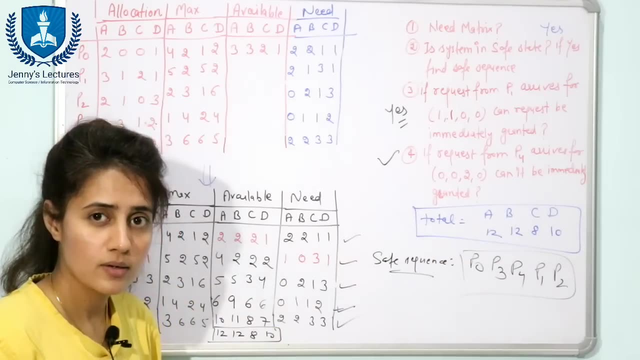 find safe sequence. system is able to find safe sequence. now you can say: yes, this request can be granted now. system will not go in unsafe state. now check out for this one. if this request comes, then can request this request to be immediately granted. same method you will apply to this also. 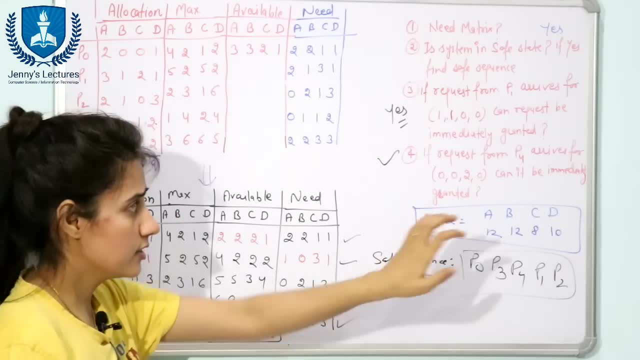 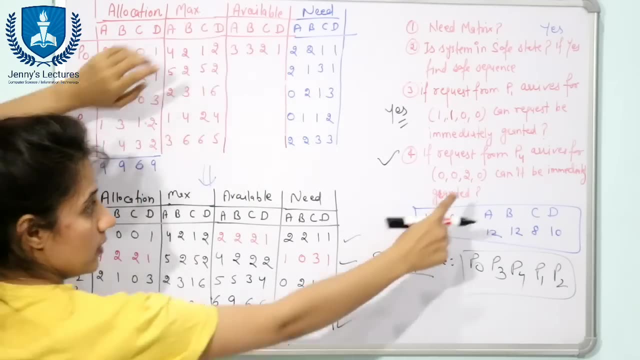 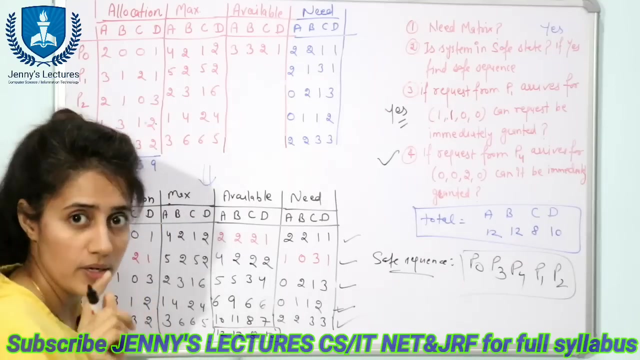 fine and system will pretend. first of all, system will pretend that it has granted this request. now, what would be the change in this case? in this snapshot, see p4- the need matrix of p4 would be changed, available would be changed and allocation of this p4 would be. 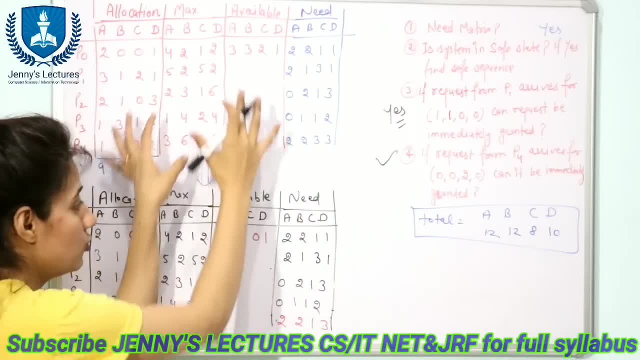 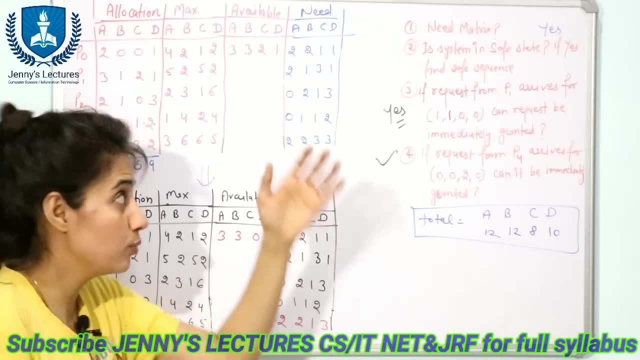 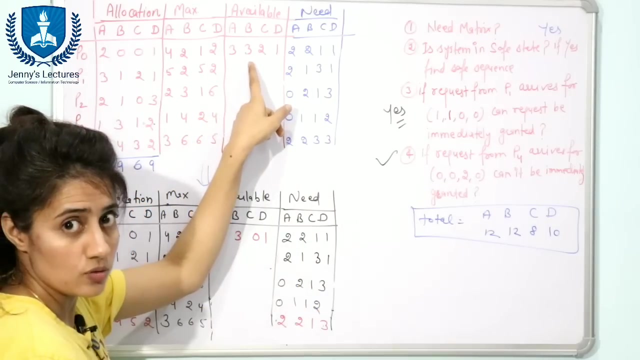 changed. now the updated state is from this to this one. after pretending that this is this, request has been granted. what should be changed in this state? available would be changed. this will will do minus of these resources from available resources. fine, so available would be one, three, three, zero and one. next thing is need matrix of this. p4 would be. 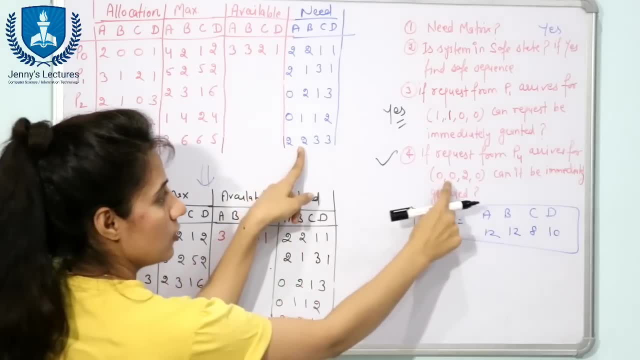 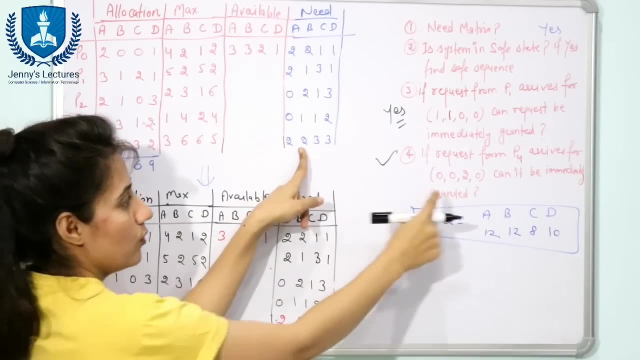 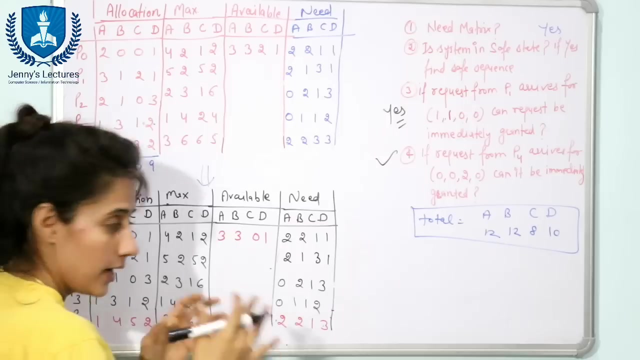 changed. need matrix is need of this before is this one and this request. p4 has requested these resources and these resources has been given to p four, so we will minus these resources to this one. so need matrix would be two, two, three minus two is one and three again. 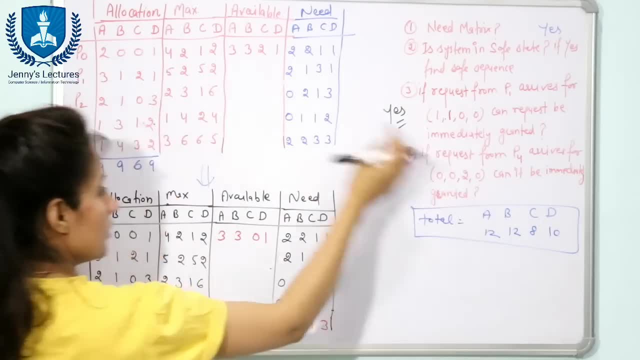 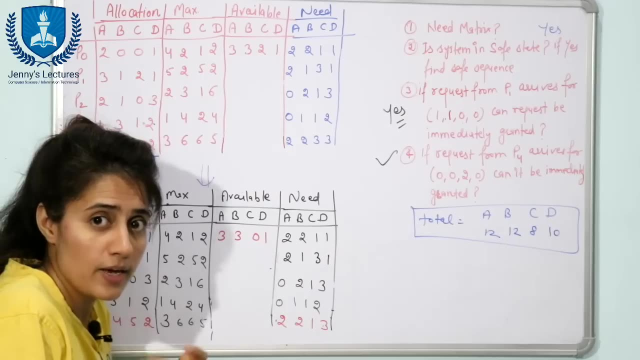 already allocated resources. are this one again located? resources are this one. so we will add this and this and this will become one, four, five and two. now, system is checking. system is applying safety algorithm. is system in checking for the safe state of this one, if you are able to find out, 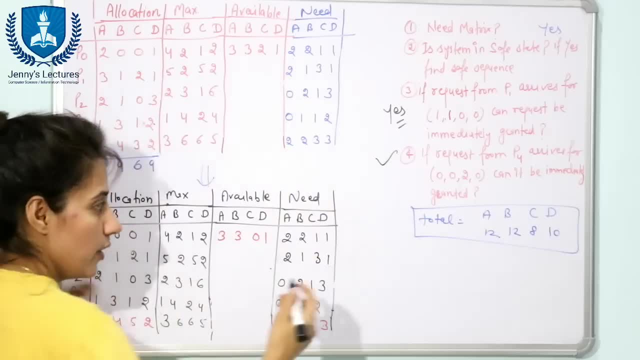 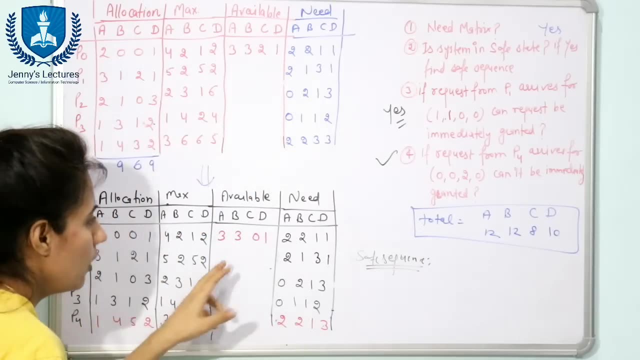 then system will grant this request. now find out safe sequence. apply that safety algorithm now, with the help of these available resources, check out which need you can fulfill. for this one, it requires two instances. we have three. it requires two instances of b: we have three. it requires one instance of c, but we have only zero. so you cannot. 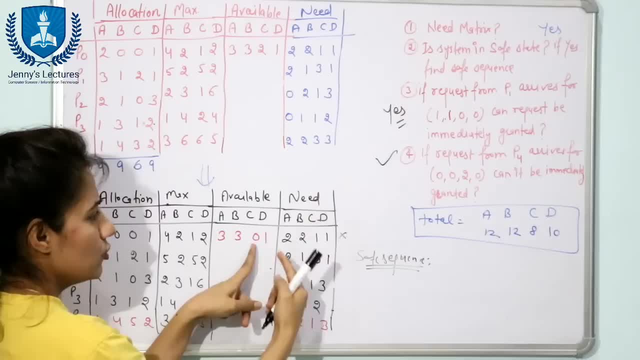 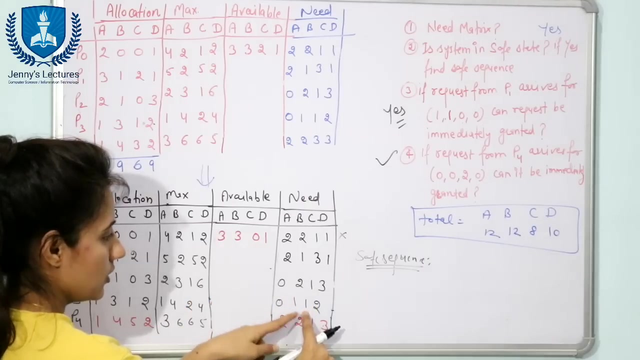 fulfill this need same with this one. so just check out for c, i guess, because available resources of available instances of c is only 0. fine, it requires three instances of c. we have 0, cannot fulfill it require. i have zero, cant fulfill it require 1 instance of c, cannot fulfill. 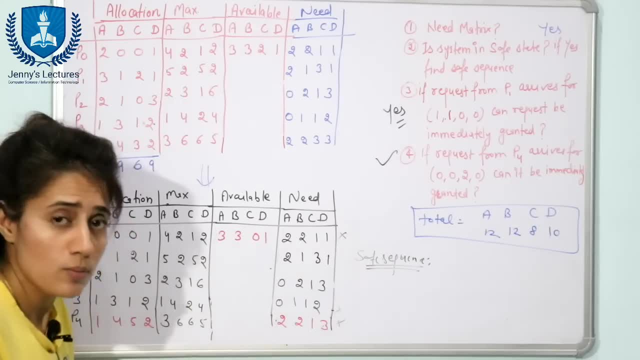 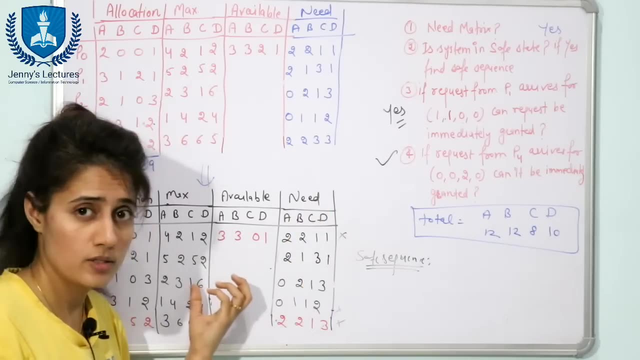 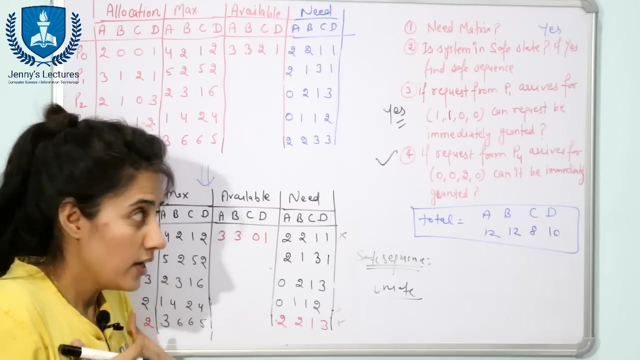 it require 1 instance of c. i have zero, cannot fulfill. so now system is not able to fulfill any process need now. obviously the system would thankful for that. so now you can see how it worked with this. data that go in unsafe state, fine, and if system find out that if i grant this request, i'll go in unsafe, 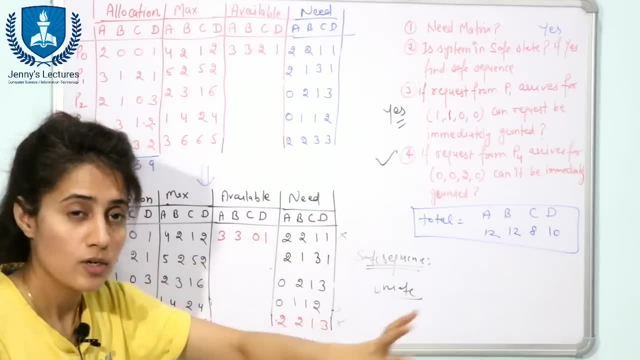 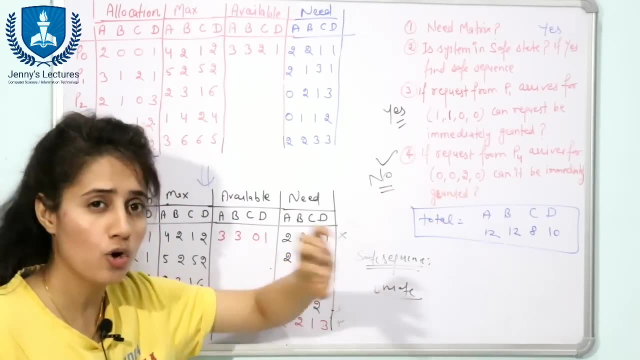 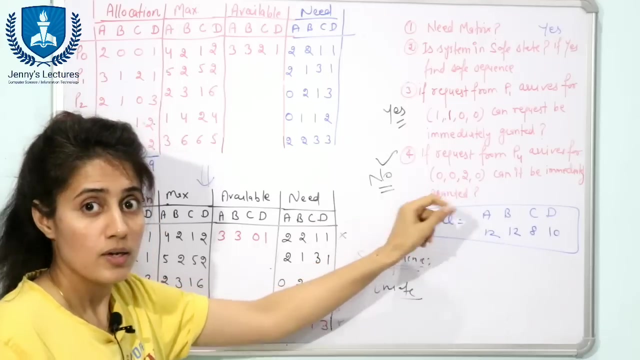 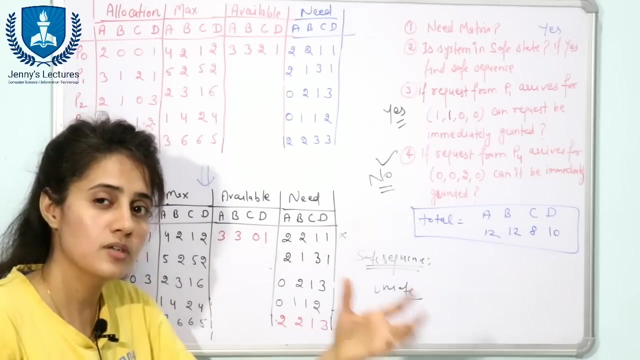 state, then system will not grant that request. so system will say no to this request. so answer would be no, this: this request cannot be granted immediately. see, although resources are available, say resources are available, so system can grant this request, but resources are available. but in future, because of this request, because of granting this request immediately, system may get. 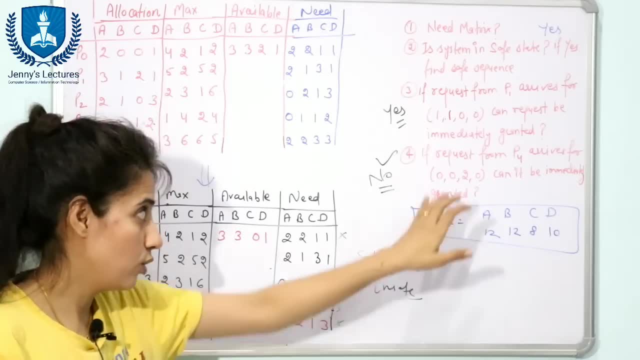 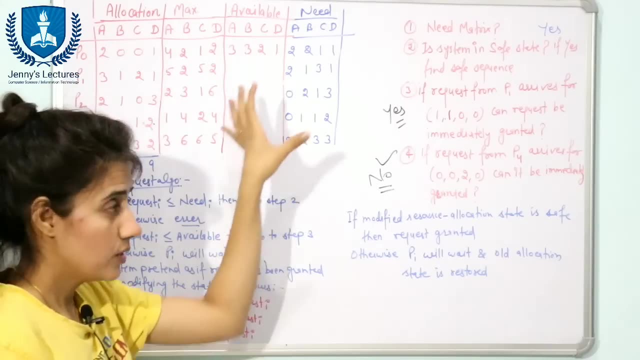 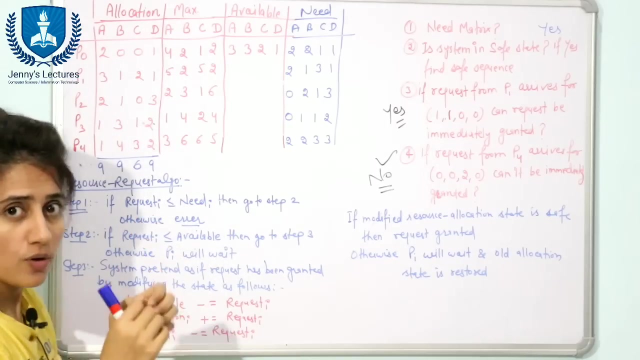 stuck, system may be deadlocked, so system will not grant this request. so this is how system will avoid deadlock. so this is a resource request algorithm. whatever we have discussed, i have written those into steps. see, first step is: if request request of a particular process is less than equal to need, then then what we will do. then what we will do. 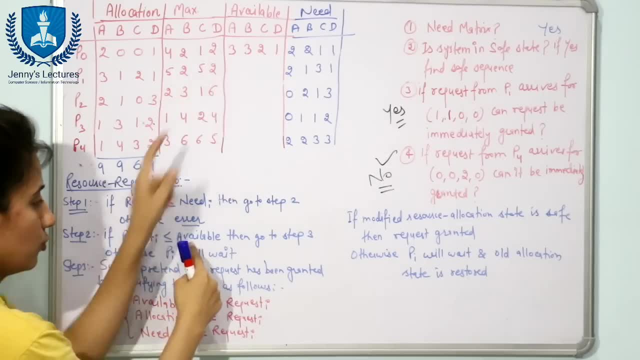 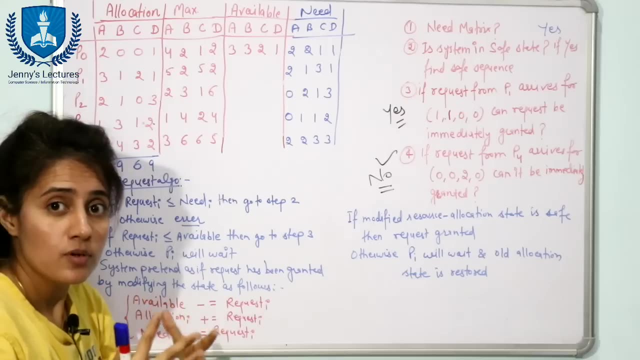 i'm going to say that if i request request of a particular process is less than equal to need, then what we will do, then what we will do again, we will check request with this available resource. if request is less than available, then we will go with step three. step three is: what system? 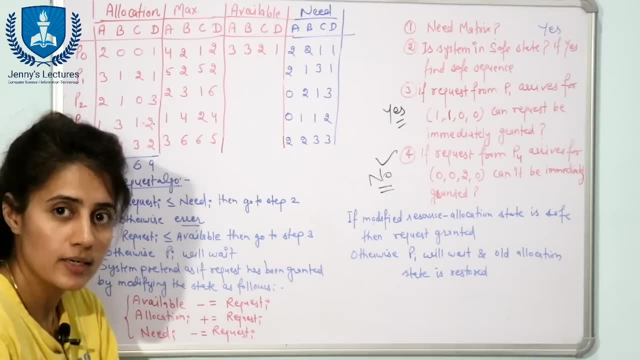 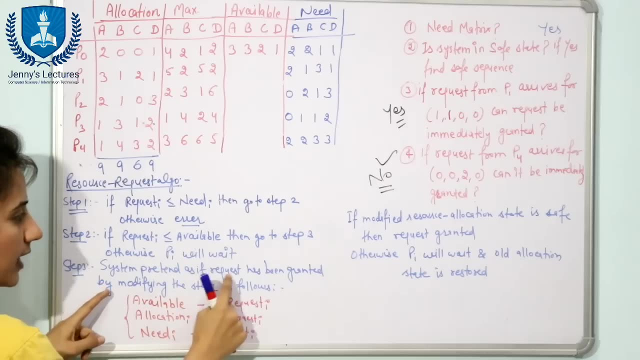 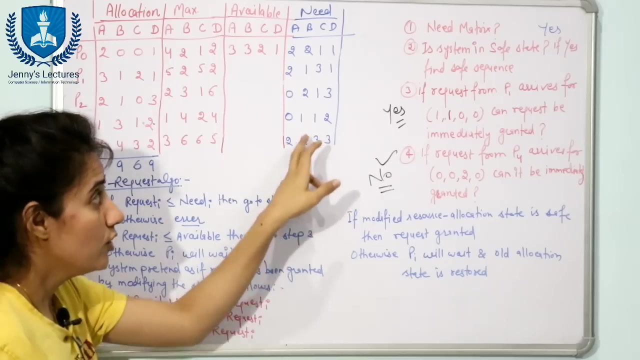 will pretend that this, that request has been granted and this state would be modified to another state, as we have discussed. so system: pretend as if request has been granted by modifying the state as follows: now, state would be followed as what need of that process has been changed, available would be changed and allocation for that process would be changed.